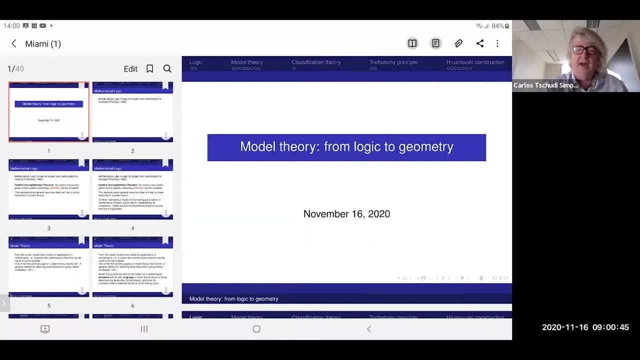 and we propose. we hope that we'll be able to propose on-site events in Miami next year. That, of course, will be subject to the to the situation. Okay, so now the topic. this of the of the conference this week is O-minimality and its applications to Hodge Theory. 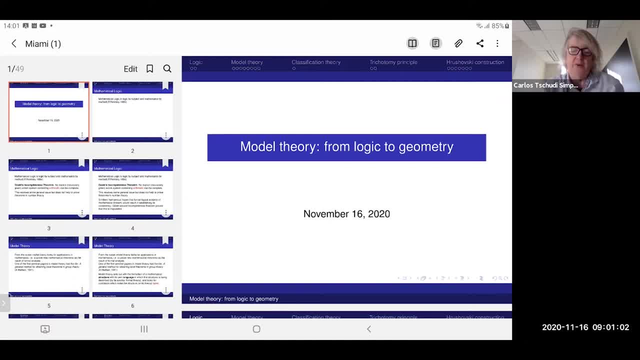 plus maybe surrounding subjects. So this is one of the most fascinating recent developments in in Hodge Theory, where logical methods are applied to obtain new and sometimes previously conjectured results. in Hodge Theory, analytic geometry and also arithmetical side of the 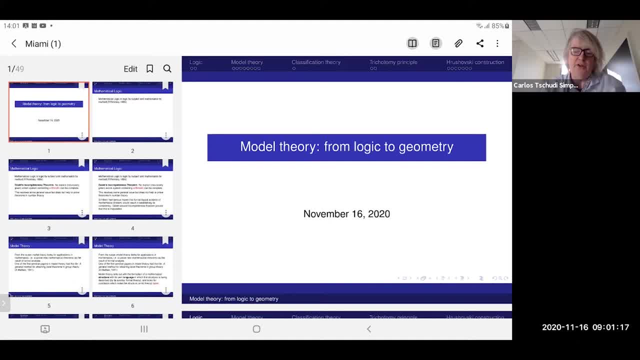 question. Okay, so it's a great pleasure to introduce to have this morning. we'll be having the start of this of the mini courses by Boris Zilber and Bruno Klingler this morning And tomorrow morning, and so our first speaker is Boris Zilber who will speak on. 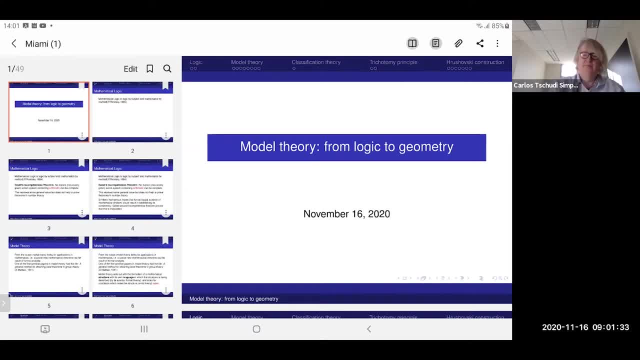 model theory from logic to geometry. Thank you, Good morning everyone. Well, I see my task as saying some general things about. well, to to broaden mathematical community to the community of geometers and maybe a few numbers theorists, to give a sort of introduction into principles of model theory and 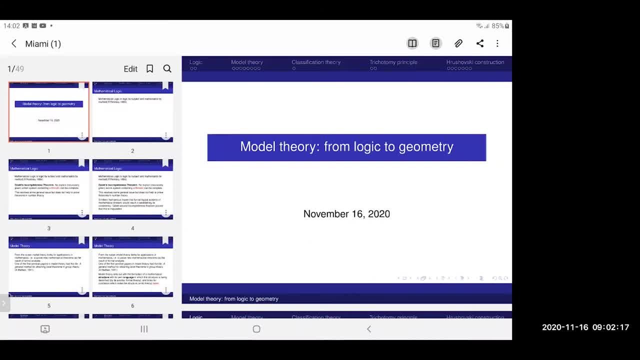 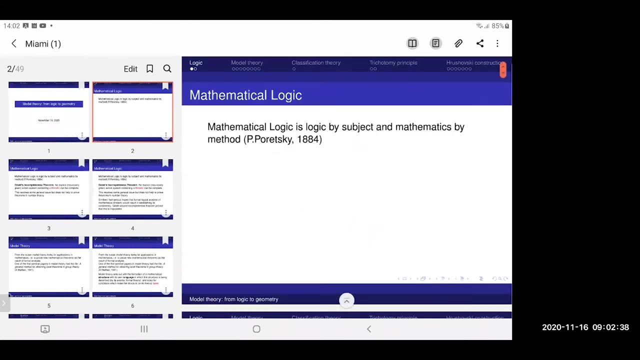 as as good as I can do this to, to explain why logic in general, once being a formal logic, um, it turned out to be useful, uh, to mathematicians. Okay, so I start with with history. So here is one of the definitions of what mathematical logic is about. 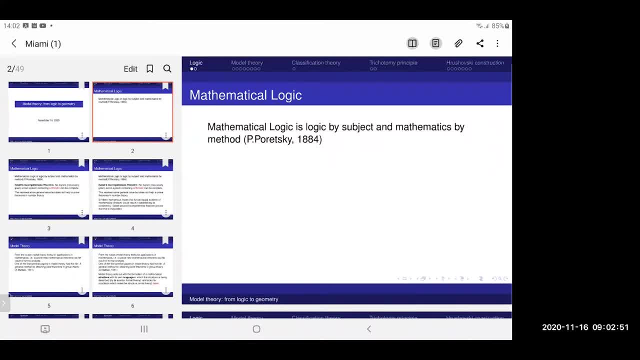 It's very old definition, but in in in broad way, a broad span, maybe in the majority of the world. Well, I'm going to start with the first one, which is theory of the gravitational direction. So if you want to know more, please go to the library online. 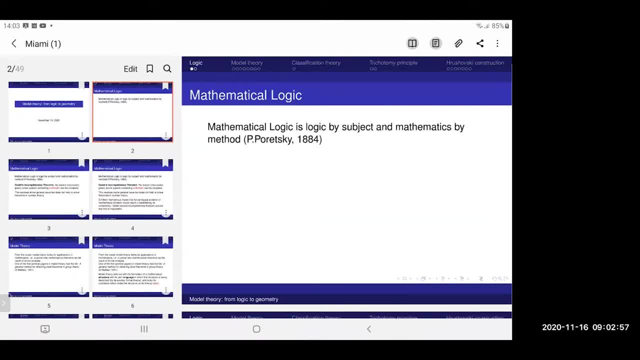 So I'm going to start with the first one, which is theory of the gravitational direction. So if you want to know more, please go to the library. online way it still stands. So it is logic by subject and mathematics by method. Now there is something. 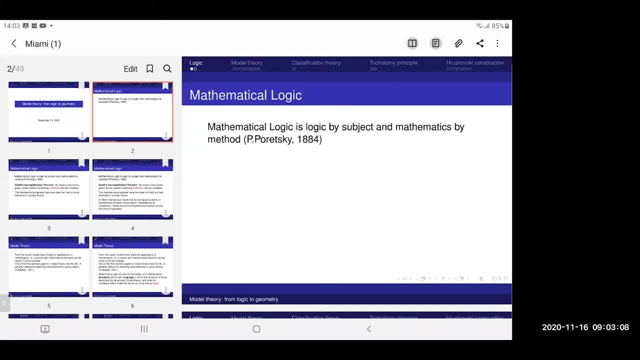 quite specific about this statement, because it is this part of mathematics which does have a subject. It is, it's almost like physics. So we start by asking questions about nature. Well, although this is not necessarily, it depends on your philosophical view of what is the source of logic, but to some people, logic is as objective as physics. So we do study. 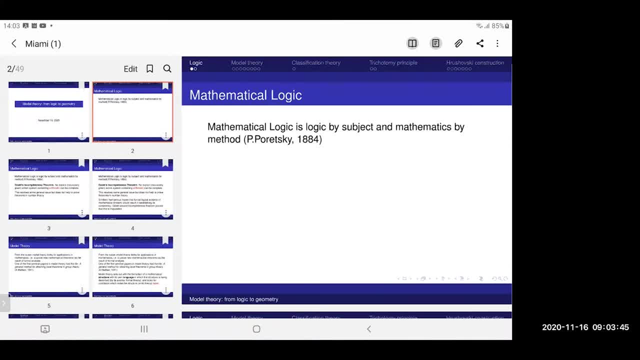 some sort of side of nature. and yeah, so the real studies started in early 20th century, and initial questions, of course, were of exactly this logical nature. and so here you see, one of the first of the two really powerful theorems that tells you that any meaningful mathematical theory 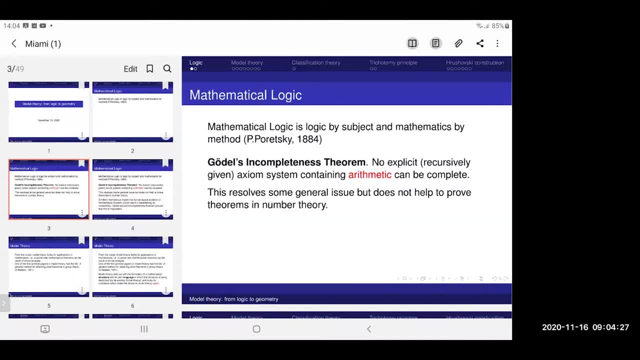 or let's say, a mathematical theory that contains at least arithmetic we cannot hope to have. We can write down some sort of axioms. There are axioms of so-called Piana arithmetic axioms, but none of this can be complete. That's the point. 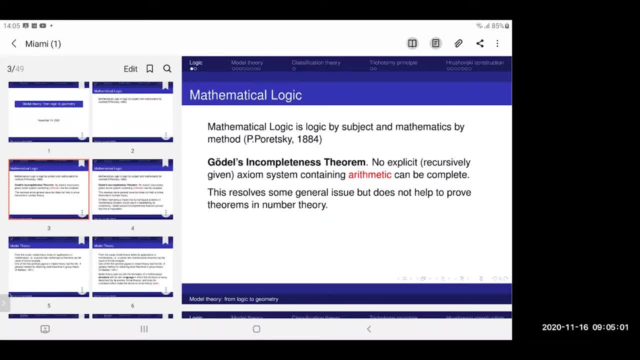 And completeness in realm of logic means that your system of axioms is such that it resolves any question, that if you feed into it a mathematical statements, then your system of axioms, theoretically, can either imply proof of this or imply the proof of negation of this statement. 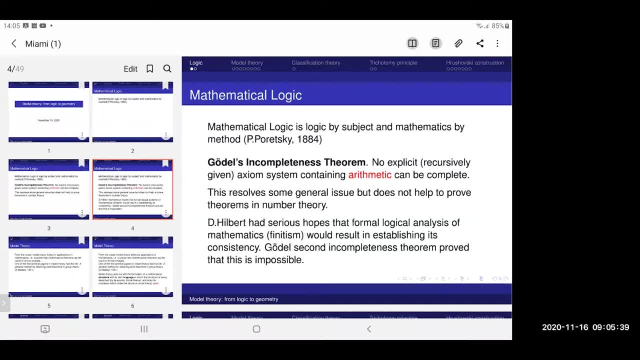 But you see, this answers some maybe deep logical question, but it does not mean that it doesn't help you to prove mathematical theories. So another, of course very important run of events at this time was Hilbert's hope that formal logical analysis would result in establishing consistency of mathematics. 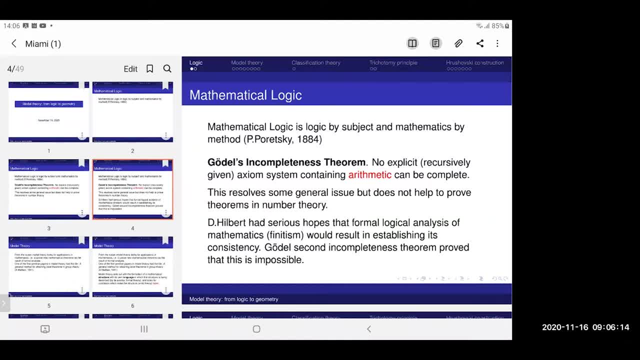 which was concern at this point, when certain paradoxes of said theory were discovered and other things. So it is old history, but it's still going on to understand in philosophical terms of what is happening here, And the second Gödel's incompleteness theorem proves that this is not. 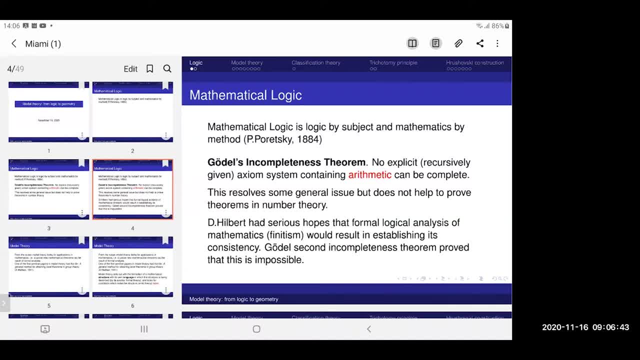 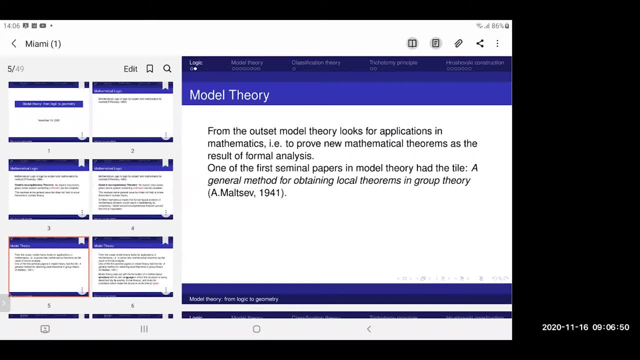 possible. Okay so, but this were pre-model theory times, So model theory came in a bit later. and here I want to emphasize that from the outset model theory was looking for applications. It was driven by thoughts about applications. It is a kind of idea that if you're good in analyzing logic, in understanding what the proof is, 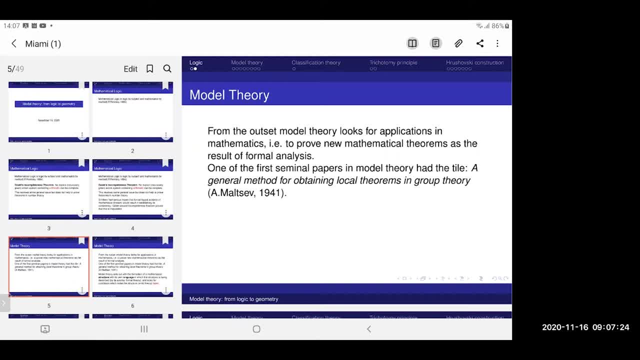 what does it mean? that it is impossible in principle to have a proof? can it help to prove mathematical theories? now, And one of the, as you see here on the slide, one of the first papers in model theory, a very important one, In fact. it also contained the proof of. 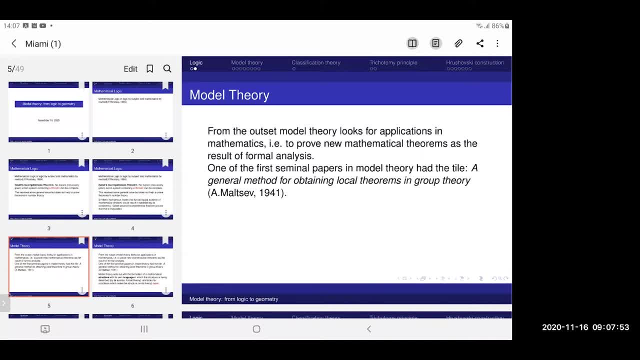 or I don't remember now, maybe shortly before this the same Maltsev approved the compactness theorem, And so this paper, general method for obtaining local theorems in group theory, was actually a kind of breakthrough paper in development of model theory. And 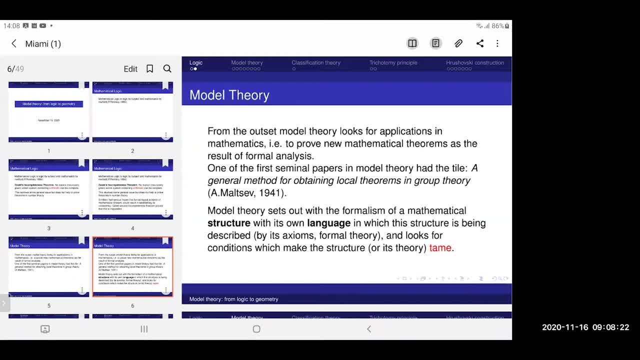 so what the model theory does, what is different with the previous times? that model theory thinks, sets out formalism is a kind of Brubakian formalism of mathematical structure. So you have a structure and the structure. you have a specific language. 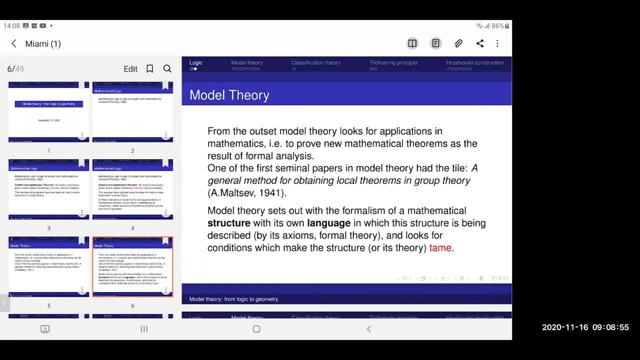 that's what determines the structure. It comes with language, and this language is actually a well. it has as its vocabulary a list of names, of relations, relations or function symbols that you allow to use when discussing this structure And, in fact, when you start with this: definitions. 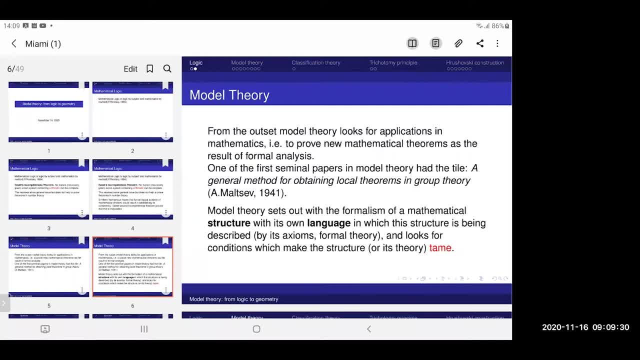 such a broad definition, you soon become interested in conditions which make the structure or its formal theory tame. So what does it mean for a structure to be tame? Why some structures are better than others? And here we have some model theory developed. 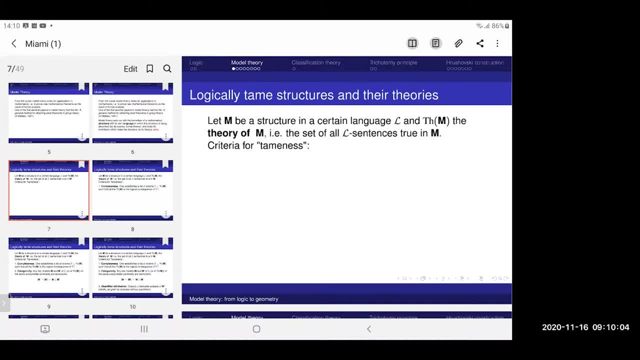 It wasn't from the very beginning but it was developed step-by-step- the following criteria for tameness- And these are rather criteria at the early stages, So I would say before 1960s, the criteria for tameness. So first of all, we already mentioned this- 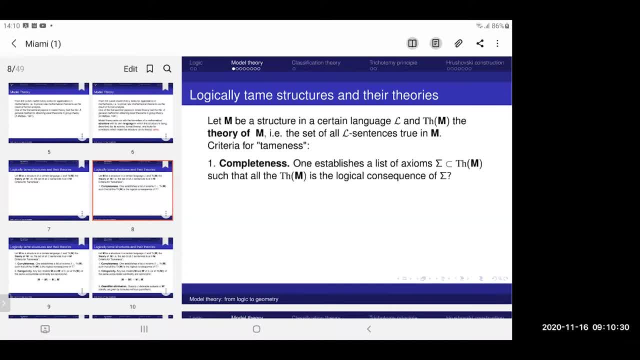 the completeness. So one looks for whether you can use this on any single point, so whether the agreement места where it must, had created. But you can come back to this to see that in mar with all the structure, And then always you need to write: 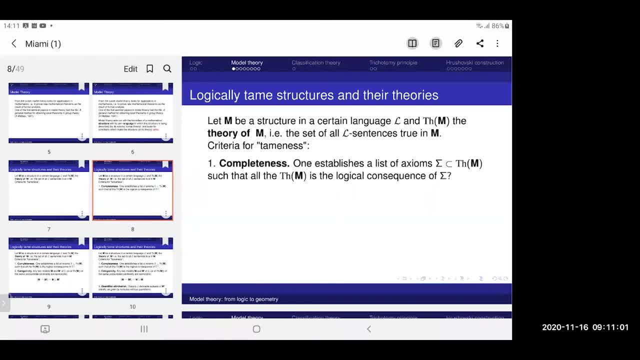 down a list of axioms, at least theoretically, a list of axioms which, of course, are supposed to be true. It is a collection of all true statements about M in this language that we have in mind. So part of this, some interesting part of the statements, forms a system of axioms. 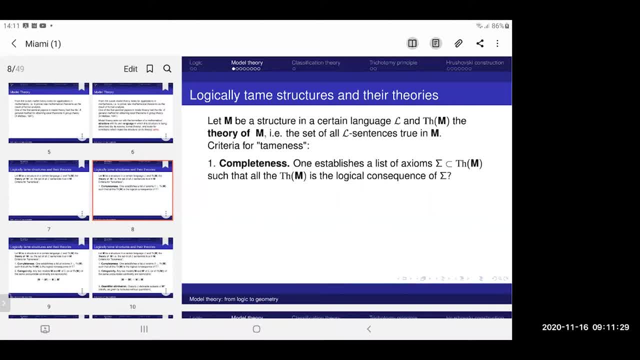 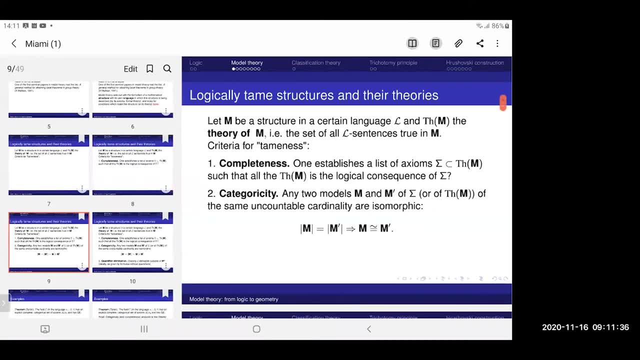 And we ask whether this system of axioms is complete in the sense that I explained. And then the next one is a criteria of categoricity. So categoricity here is the old word which has nothing to do with category theory. So the definition of categoricity is: 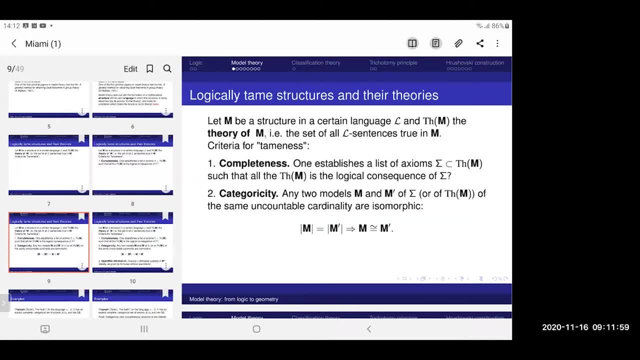 It is that you have your axioms. you have such system of axioms that it is so complete that it determines your structure uniquely, up to isomorphism. So it is stronger than completeness. So the theory is so strongly characterizes your structures that it is categorical. 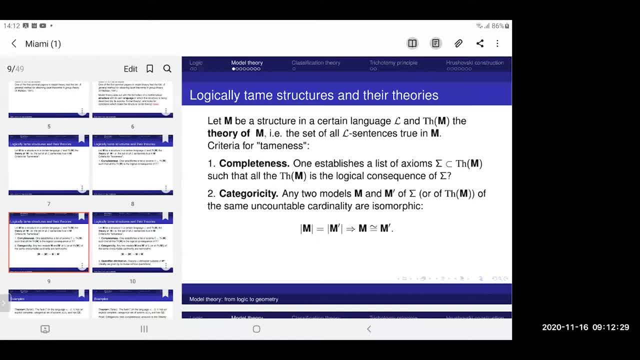 It is categorically characterized. By the way, about the same time when logicians discussed this notion, maybe a bit earlier, a physicist also discussed the very same notion, but in terms of Well, they called it univocal. So they discussed with their theory of physics. 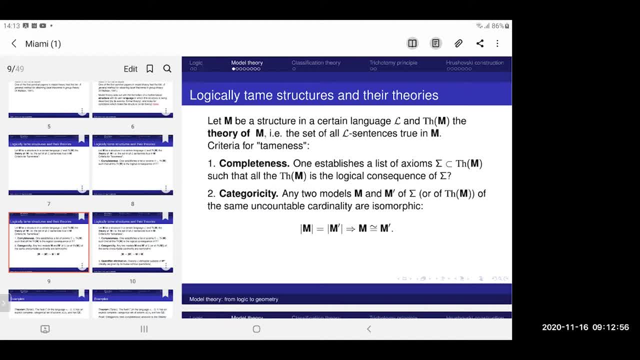 And Einstein was very Seriously involved in this discussion with the theory of physics- should be univocal, So that it defines, it determines unique model. we would say. So categoricity, again, is a stronger assumption than completeness, And in fact, well, here you see, it is important that. 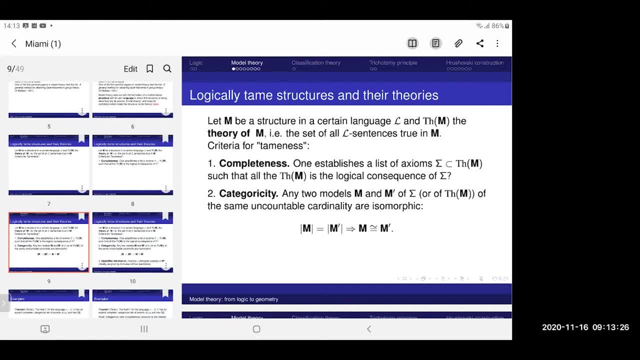 In this definition. Okay, In this definition. well, I narrowed my definition, my version of this definition, to consider only uncountable size of the structure. Well, you can, without any problem assume that we are talking about continuum, the size. 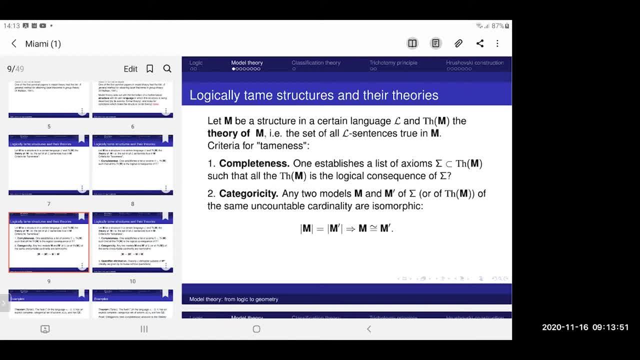 of the universes, of our structures, to be just continuum, like field of research. Okay, Okay, Thank you, Thank you, Thank you, And I think that the question is- well, let's go back to the expression- that there is no. 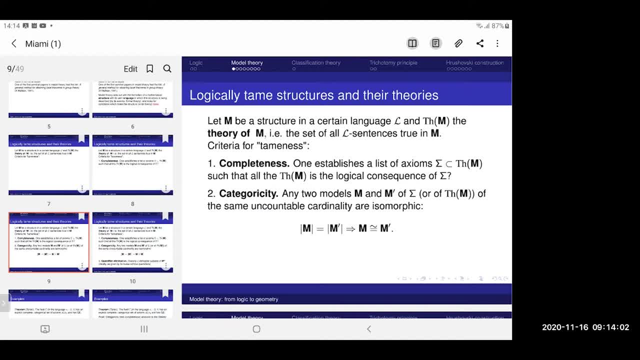 real numbers or field of complex numbers or any usual geometric object, And actually it doesn't matter whether it is continuum or any other uncountable cardinality, as was proved by. So it was a great theorem that started this business in series by Michael Morley in the 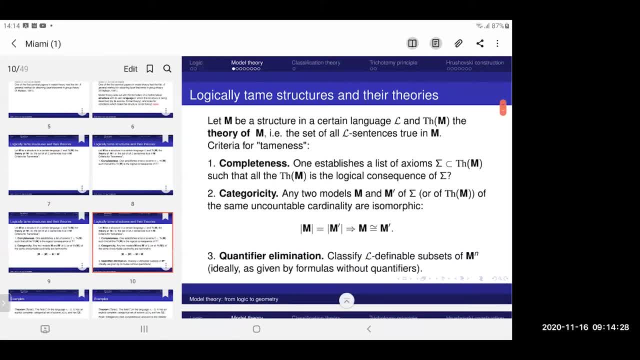 1960s. Okay, and then the third assumption, the third condition that we look at when we study a theory of a structure is whether we do have a classification of definable subsets. And I'm going to give quite a few examples, but before even I go towards these examples, you see. so what typically is a definable subset of? let's say, you have affine space, say, over the complexes? 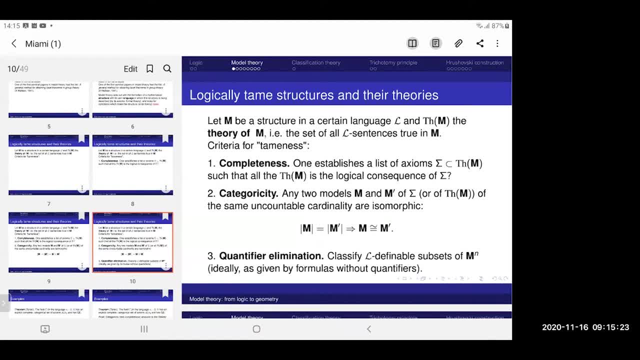 and what is definable. if you only use addition and multiplication, You can write down an equation, just usual polynomial equation, and by this you define some curve or surface or some such thing, and this is the typical definable subset. But because we are talking about this logic, 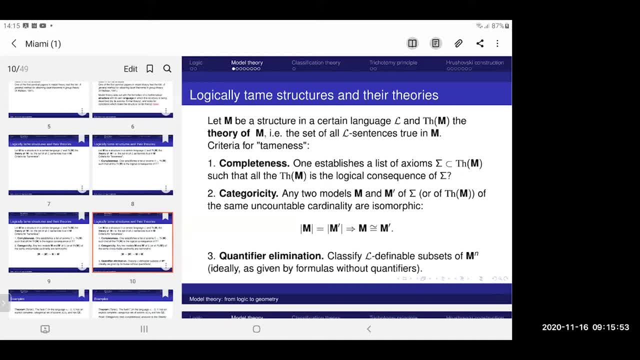 there are some logical languages that also allow not only write down equations or negate these equations and take conjunction between them, but you can also use quantifiers. You can say: for all x, I should be able to find y, such that y squared is equal to x. 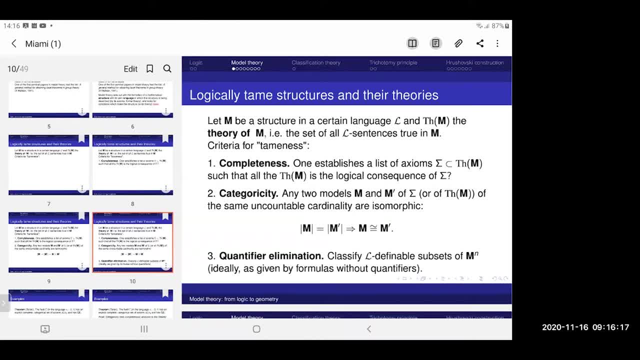 So this sort of property, So you can Express it without quantifiers, And so you have much more power of definition, And so you want to classify this. So what are these definable sets? And quantifier elimination theorem is one way of saying that, in fact, you can reduce any such definition. 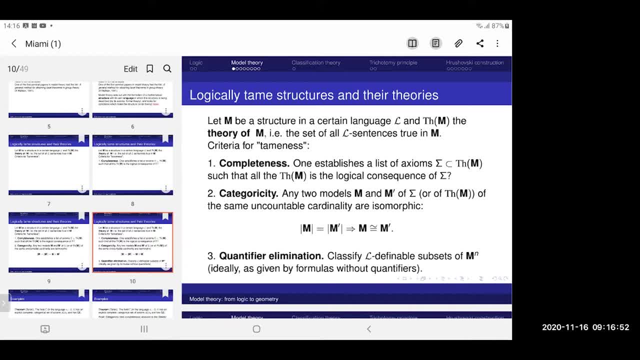 That I started to formulate to a definition that is just a combination of very simple expressions like equations, negation of equations, So something that doesn't require quantifiers, And this is called quantifier elimination, But in principle, in many examples you see, it is. 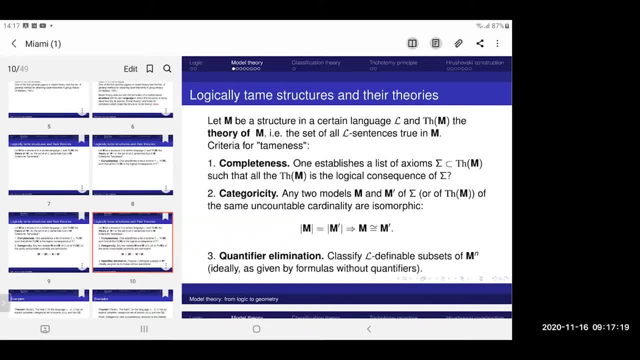 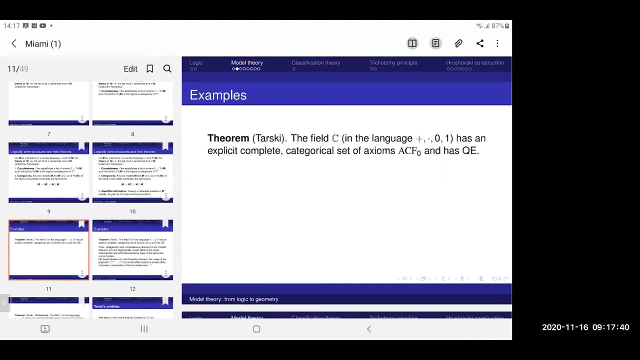 When I, When- we use this criteria Number three, We could be satisfied with a little bit less than quantifier elimination. You would be satisfied with some sensible way of classifying definable sets. And now we go to some classical examples. So this is: 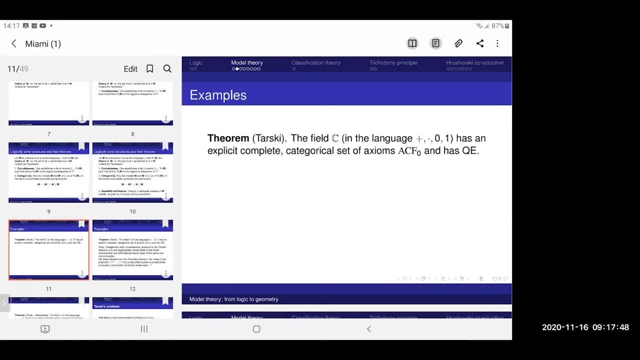 A very old theorem of Tarski. This is: this is another beginning Of Of The Trend in model theory. Let's go there and look at structures One by one and apply those criteria. And so Tarski, I think it is late 1940s. 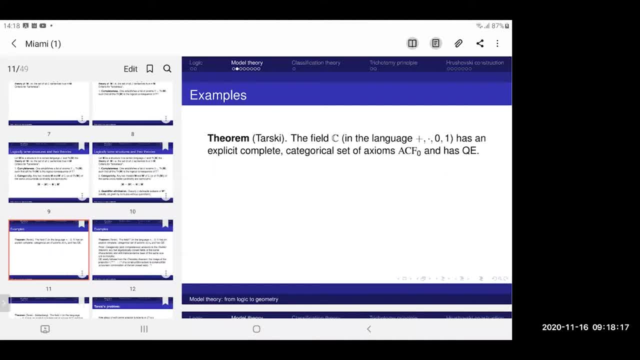 And this is Proved, that If we Take the field of complex numbers Or in fact Any algebraically closed field Of characteristic zero, So I I use here characteristic zero, Notation, Well, assumption, But in fact the same true for any algebraically closed field of. 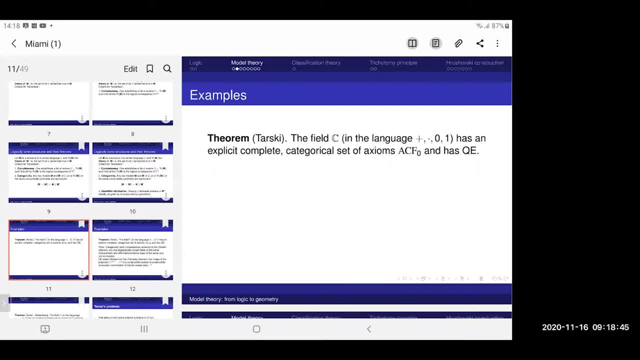 Any characteristic. So in this very simple language, where you only use addition, multiplication, You also have zero and one And when. If you have one, Then you can build two, three, four and so on, And, and, and, and also. 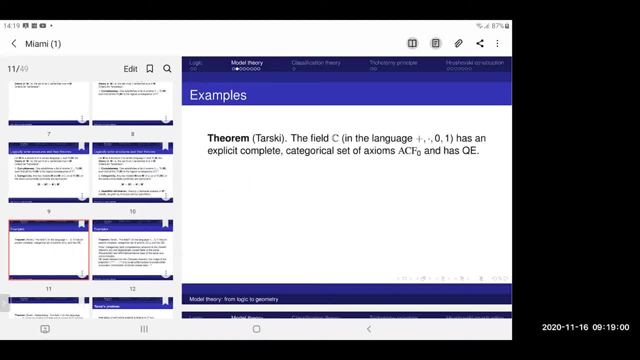 Rational numbers. So you can use all this is, As your Named, Coefficients in your polynomials And You can also say That There is A coefficient, An abstract coefficient, which can be any Complex number, and so on. 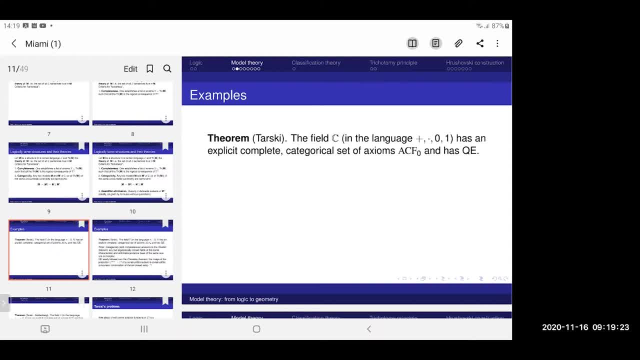 So If you Work in this language, With this structure, Then The answer is very nice That you have Complete, Well explicit Theory can be written down. It is quite obvious what you Need to write Down. 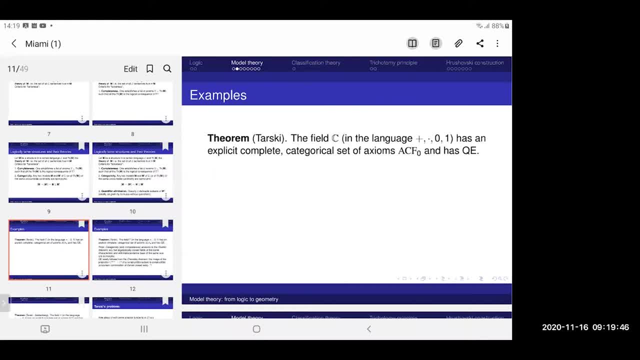 Here. But It's not only complete, It is also Categorical And has a quantified elimination, Which in this case means exactly that. It is Just Very simple formulas. And And now the proof. The proof is actually. 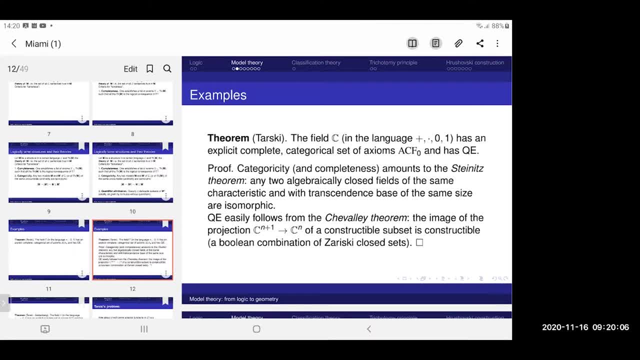 Rather straightforward How we do it today. So So one: Once you establish Categoricity, You also establish completeness And Categoricity Amongst Two Well-known Steiner's theorem That says that Any two algebraically 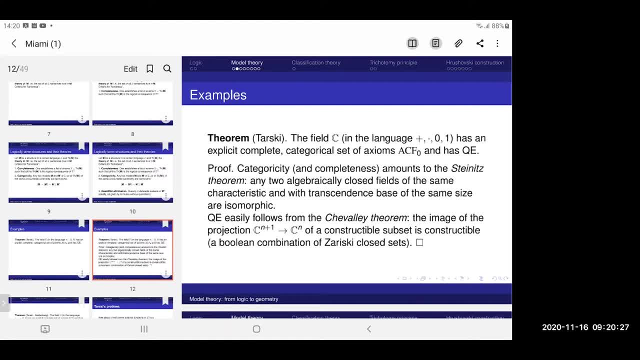 Closed fields Of the same characteristic And with The same Size Transcendence Base Are Isomorphic. So it is A basic Factor Of The theory of fields. Now, Quantified elimination Is: 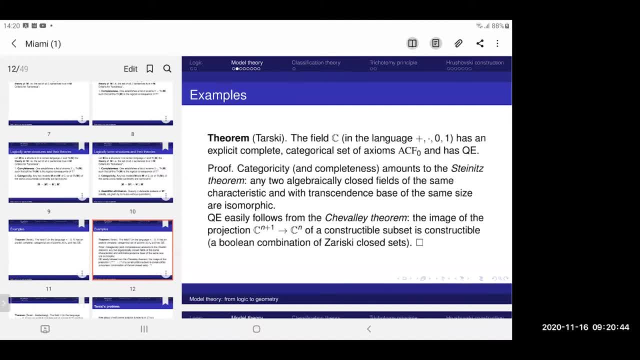 Just A little bit Trickier, And In fact It is The same argument It is. It is In fact The- Again Well-known To algebraic Geometers, So-called Chevalier. 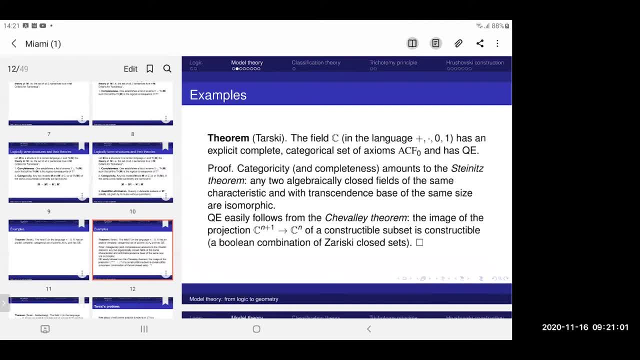 Theorem That You need Just To understand What Happens To The Image Of A Subset. So What Is Constructible Subset In The Language Of I? 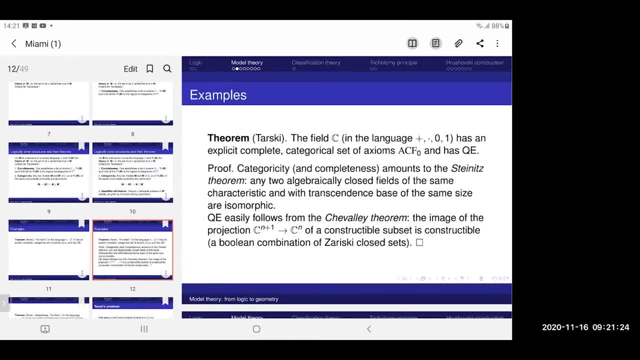 Think That Algebraic Geometers Use This Language. So It Is Just Bullion Combination Of The Risky Closed Sets Of The Existential Quantifier. So 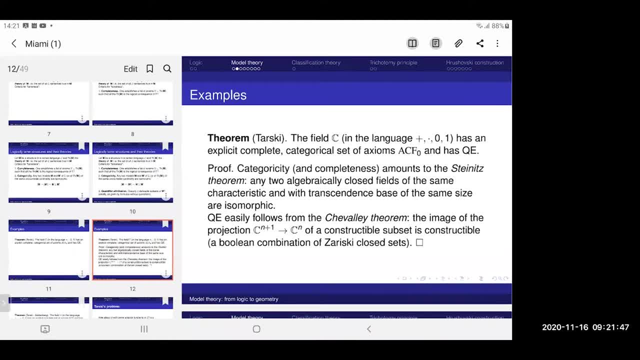 So This Is? This Is A Classical Trick Of- Well, Not Trick. It Is Classical Way Of Eliminating Quantifier, Just To Understand What Happens. 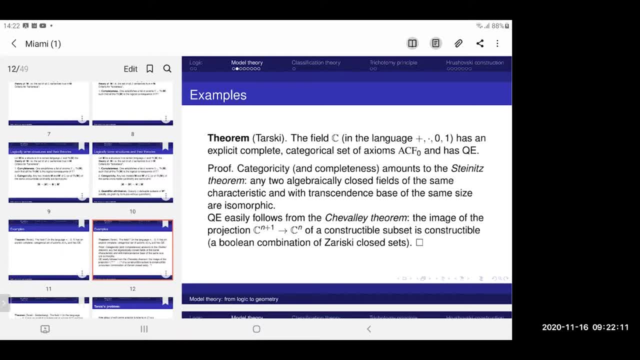 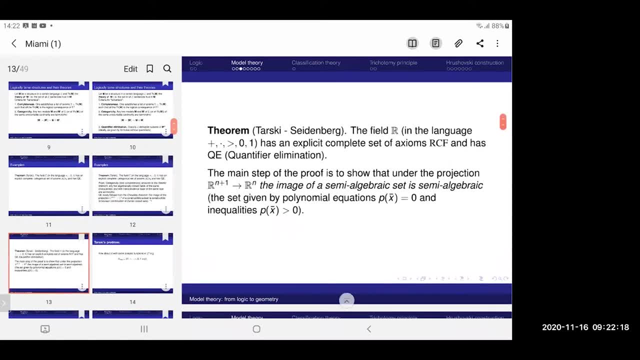 To In Terms Of Existential Quantifier And Negation. So No Problem Here, Right Next Comes A Bit Trickier Theorem, So It Is Referred. 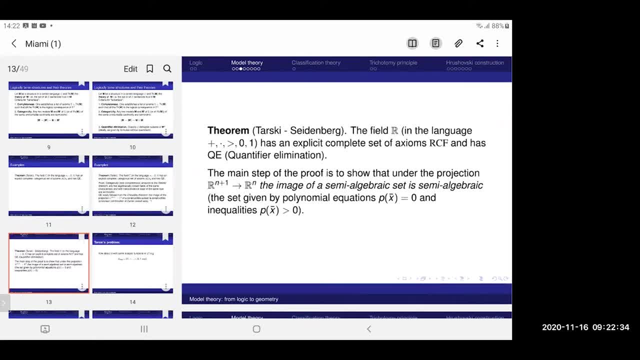 To As A Task Is Right In There You Can Say It Is Completed. So The Axioms That We Usually Refer To As Axioms- 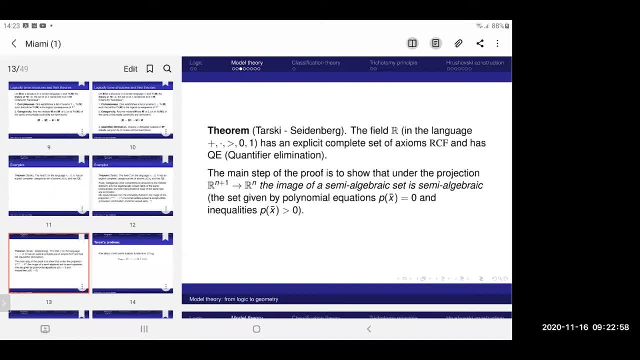 Of Real Closed Fields There Be Trickier And I'm Not Going To Go Anywhere That Between Two Values With A Bit With With Different. 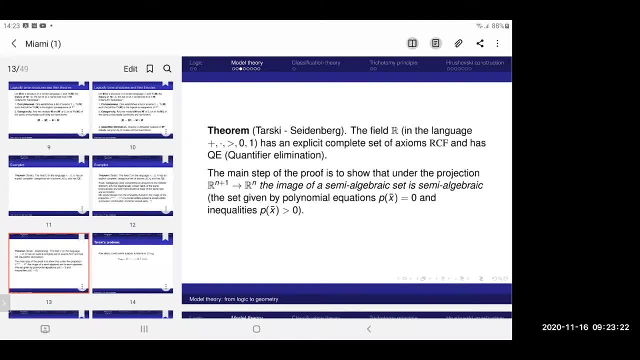 Sign Of A Polynomial. So If You Have A Polynomial With Two Different Values, Then Between Them There Is A Polynomial Of Quantified. So Again, 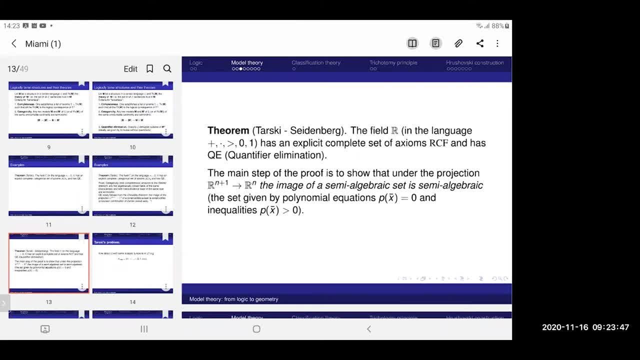 The. In Fact It Is. It Is Very Close Analog To The Statement That, Very Close Analog To Chevalier. But Now You Have To This: 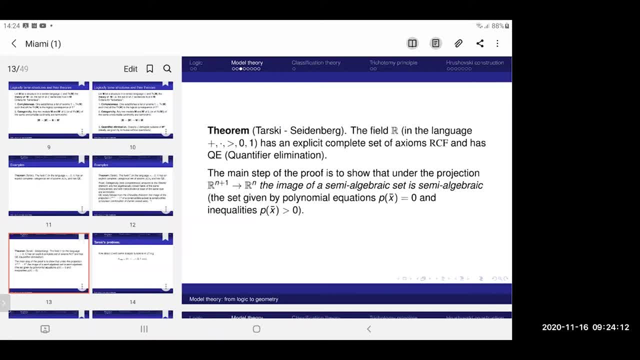 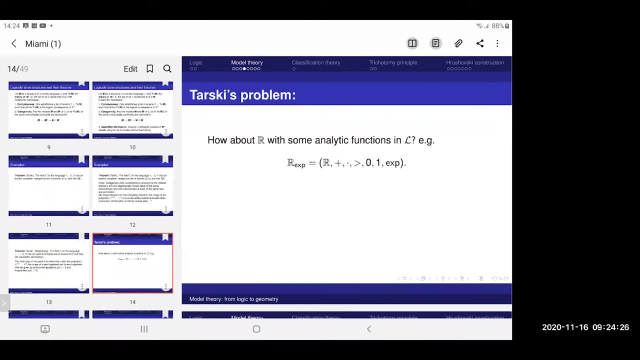 Very Natural Thing That I Guess That Many Geometers Are Familiar With. So The Notion Of Semi Algebraic, And It Was Starsky Who 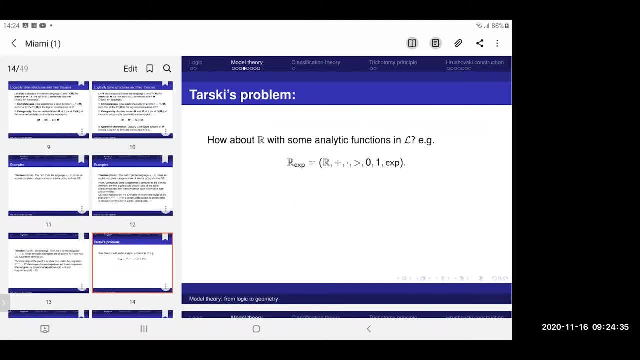 Who Then Went Further And Asked The Question Of What Is The Real? And We Do. We Are Allowed To Speak About Reels In Terms. 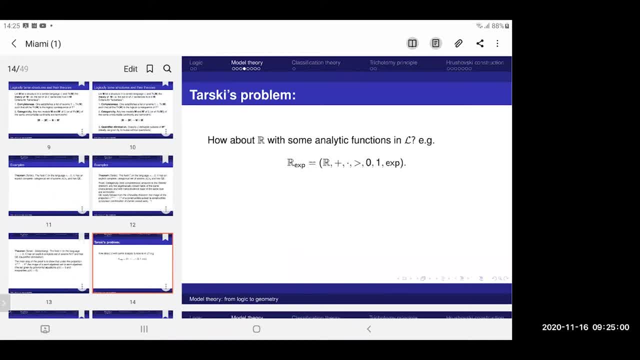 Of In Algebraic Terms, In Terms Of Addition. Multiplication In Equality Is A Theme In Fact. Well, Starsky Actually Asked This In In More. 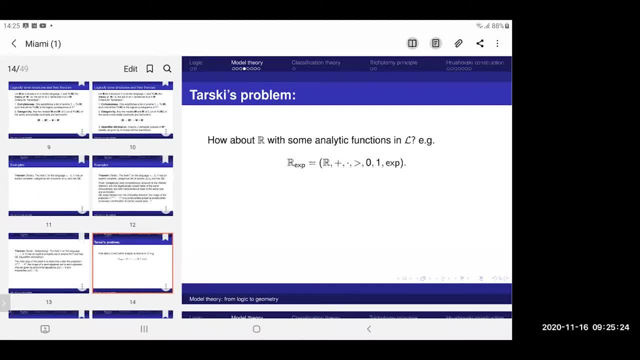 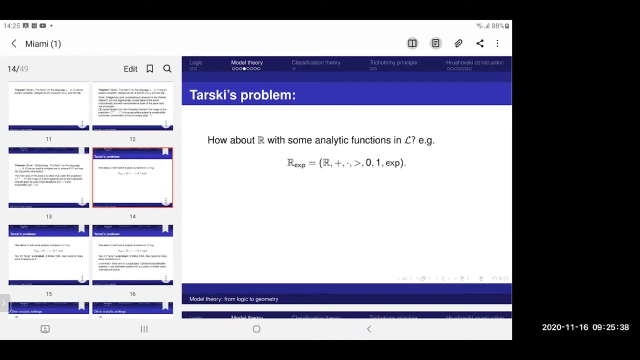 Specific Logical Terms, This Question, But The Way That We Understand It Now It Is. It A Modern Times? Well, It Was Celebrated. Theorem Of. 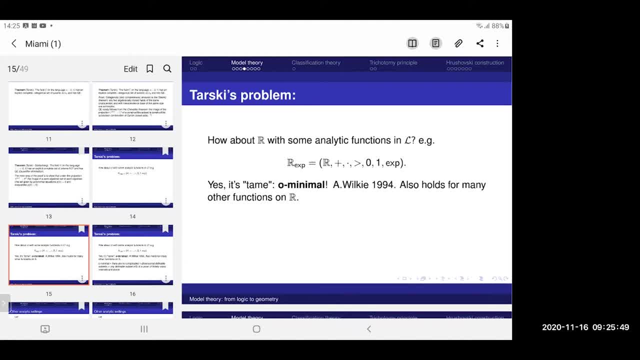 Alex Wilkie It. It Was Very Difficult One Actually. This This I Guess It Started They Did Working On This Andres Walked Worked On. 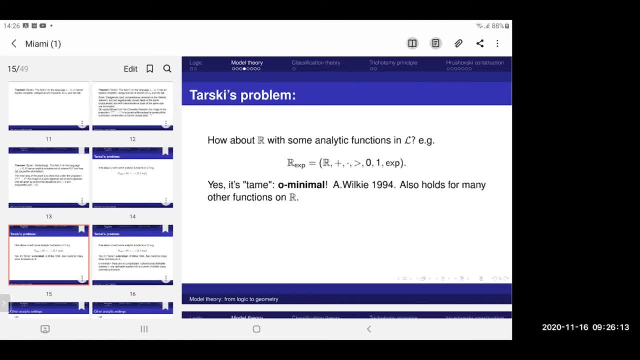 This And Well, Alex Was There From The Very Beginning, So And A Lot Of This Work Was Was Was Just In On The Scrapping. 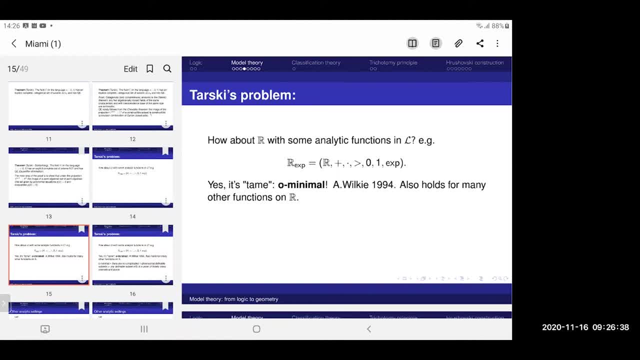 This- Alex explained this in his talk for Burbaki seminar- that the actual breakthrough to this came after it was formulated the condition of tameness, which since then we call hominimal. So hominimal is an abbreviation for order minimal. So all hominimal theories have this inequality sign. 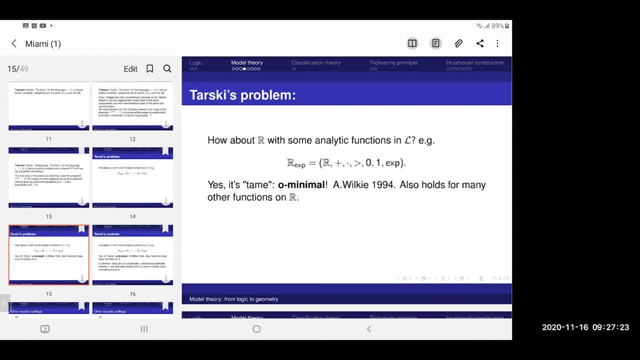 in the language And, sorry, So it is. so this, this is really so. the idea of minimality, it actually came with the, so here is the definition of hominimal in some very short form. So so the idea is that. 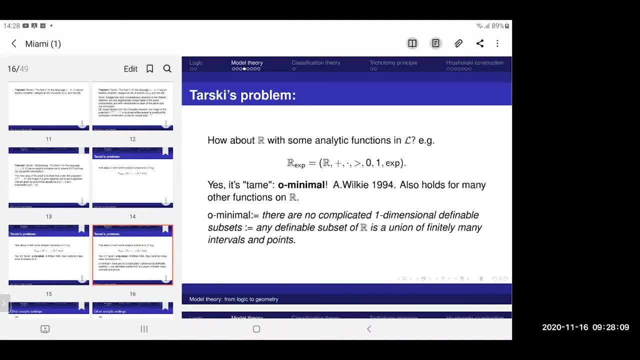 in hominimal structures you can. you can classify very easily one dimensional definable subsets, So there are no complicated one dimensional definable subsets. or, to be very precise about this definition, that any definable subset on the real line is a union of finitely many intervals and points. 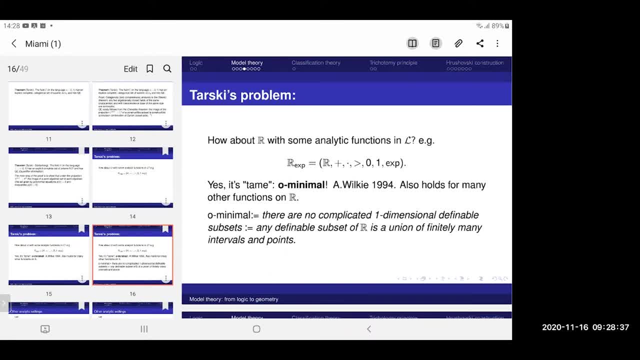 But you see this, But this is the definition which was without the term or minimal, which was originally- was realized that the usefulness of this by love and injuries, in 1986, I guess. And then Pille and Steinhorn, they compared it with the developments, with Morley's theory. 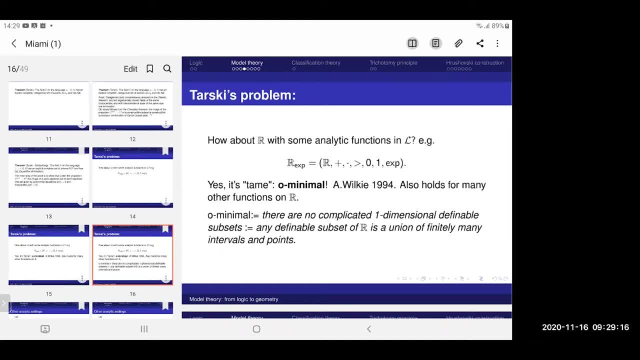 of categoricity, which used the idea of one dimensionality in terms of strong minimality. So they came up with the very abstract idea of what, of this definition? Or minimal, where it is not necessarily the reals. you should be talking, we should be. 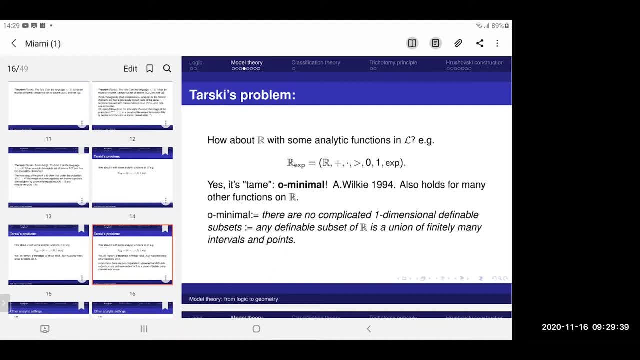 interested in but any ordered structure. So we have kind of a linearly ordered set And on this set some structure sits, and in terms of this structure, in terms of the language of this structure, You have that any definable subset of the line is a union of finitely many intervals. 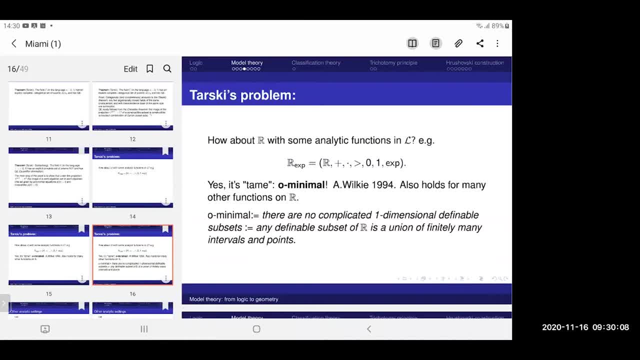 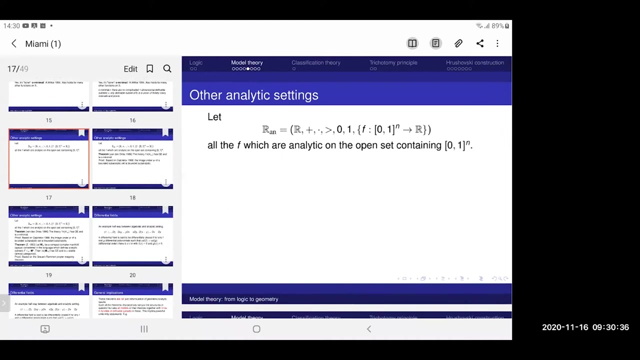 and points And they started to develop a general theory in analogy with the theory of categoricity and stability, And it turned out to be very useful for eventually that Alex found through technical proof of this, And so now we have many, many more or minimal structures, and I'm sure that Bruno, in his 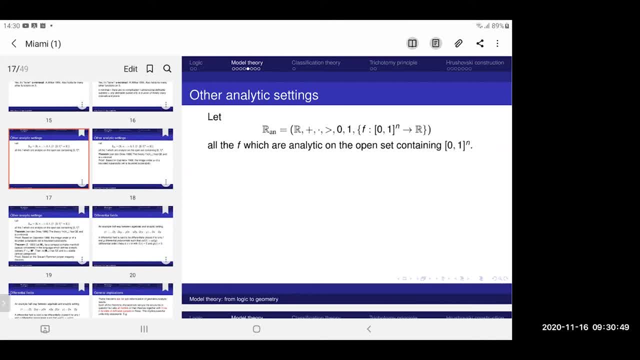 lectures will say much more about minimal structures and give more details, But so I will continue to talk about principles rather than these details. And here is another very important structure on the reals that has an analytic nature. So So now what we have is 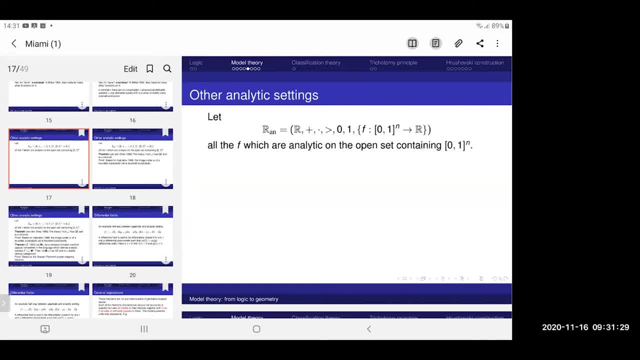 So we pronounce it R-an, And so what we have? we have the same field of Rios, but now you have name, and so you can use this name to write formulas for any bounded analytic function. So it is supposed to be analytic on an open set which contains the cube. 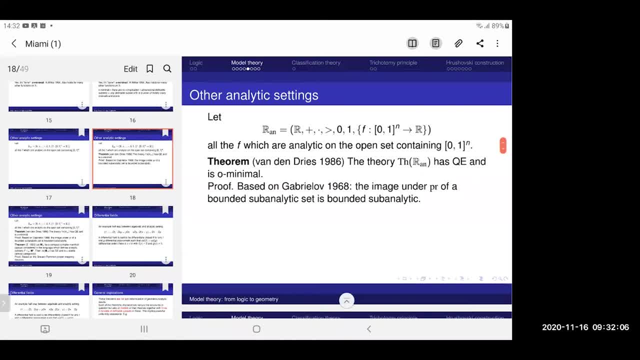 And so what we have this is this theorem of Van den Rys, where he already talked on this property of minimality on the real line, And so this theory has elimination of quantifiers and is for minimal, But in fact, as Van den Rys explains himself, so all that he needs to do is to understand. 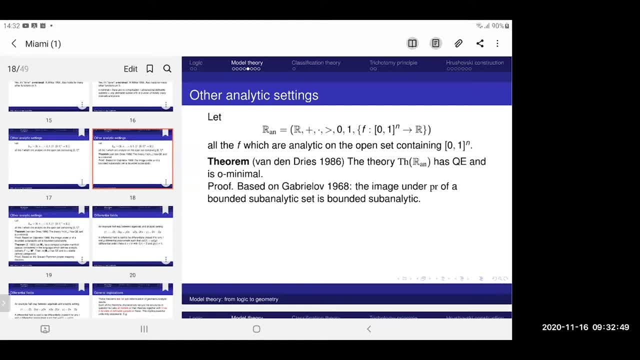 and apply Gabriela's theorem, That of 68, that image and the projection of a bounded subanalytic set is bounded subanalytic. So again, it is an analog of the Chevalier theorem. so we need to understand what happens. 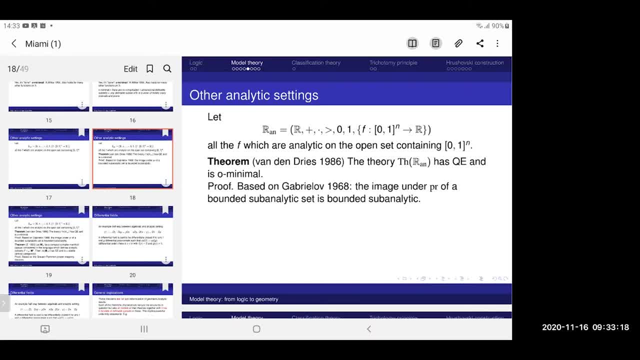 with a typical definable set. So typical definable set Here is bounded, subanalytic and well, not exactly true that all are of this nature. So you have a combination of bounded subanalytic sets and unbounded algebraic sets. 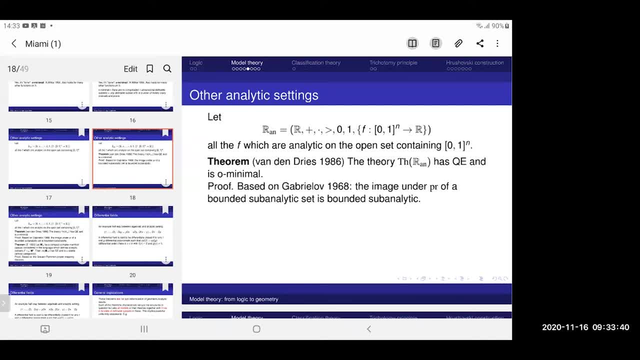 But this one is enough, and then it is a technical work of Van den Rys that makes it work. Okay, And now let's see. Okay. So now, here is another thing that I noticed in some years later. So coming not from the reals, not from the interest in structures on the reals, but rather 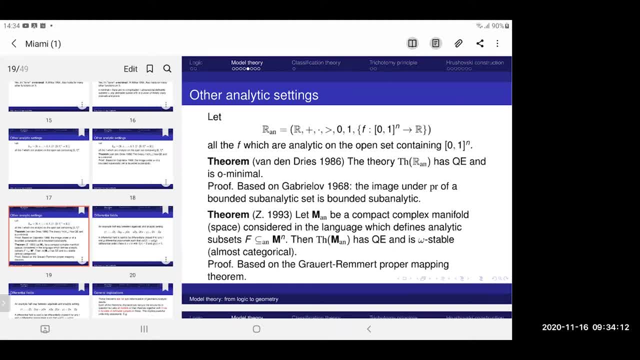 from the interest of the other side of moral theory, this stability theory and categoricity, And it is always the context of complexity And it is always the context of complex algebraic geometry Or, in this case, it is the context of complex analytic geometry. 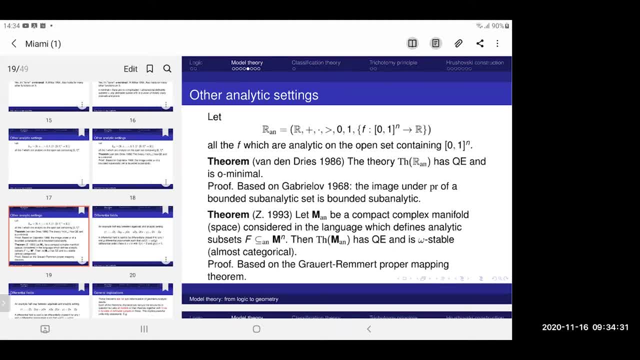 So the fact that I noticed it is that if we construct a structure, if we pick a structure, the universe of which is a compact, complex manifold, or even a compact, complex space, it would be the same argument And consider it in the language which has names for analytic subsets on the Cartesian. 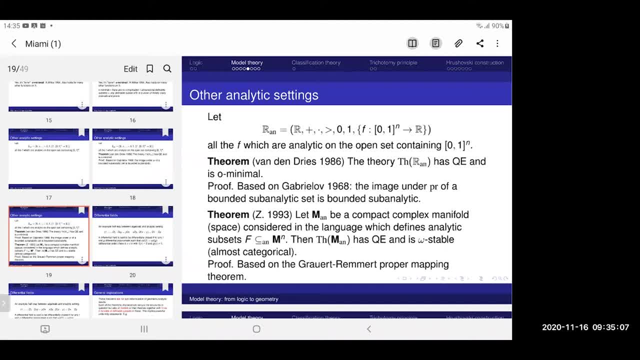 powers of this, Then this structure has actually quantified elimination and is what technically we call omega stable. But it is not. But even more, it is almost categorical. Well, almost categorical really means that you can decompose it into some sort of connected. 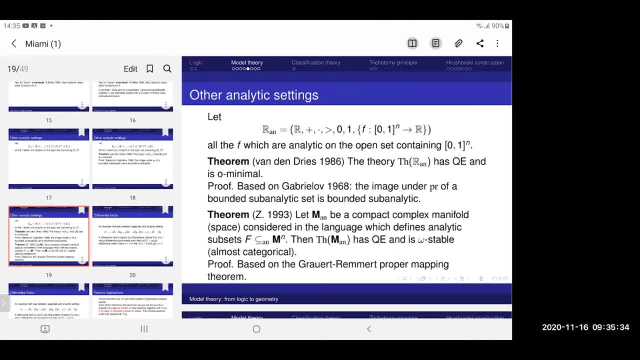 components which are categorical. It is a bit imprecise, but that's a good way of thinking about this And I'm using this term on some of my next lectures. So I'm going to go back to the slides And, as you see in the slide, this theorem is actually again the proof of this theorem. 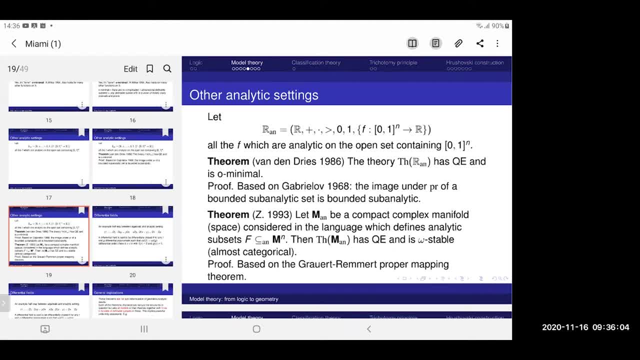 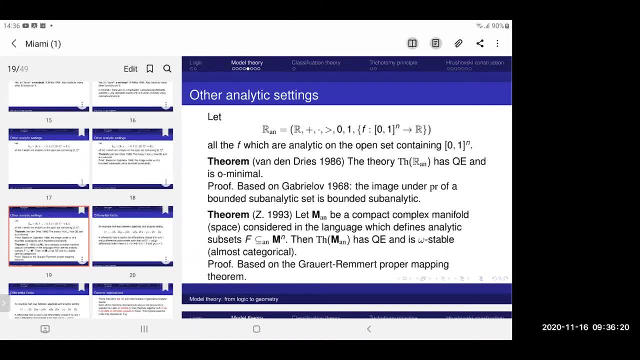 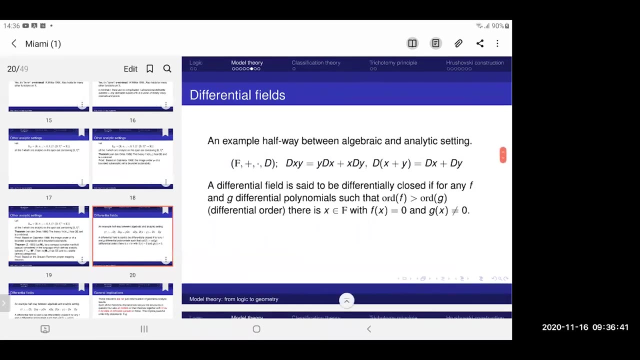 many in the world of analytic structures There are some that are also very thin. Okay, It is Grout-Remert, proper mapping theorem and a little bit more. Okay, Right. So here is also quite an important form in model theory and applications example. 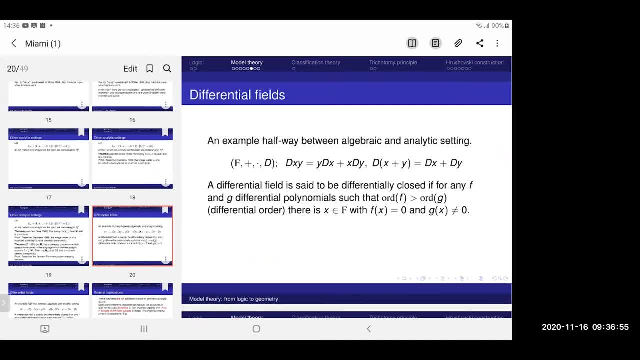 which we usually see as something that is between algebraic and analytic setting. So you really have a field, So formal structure, you have additional multiplication and you have a differential operating that satisfies this Leibniz rule. So in what you see in this slide, 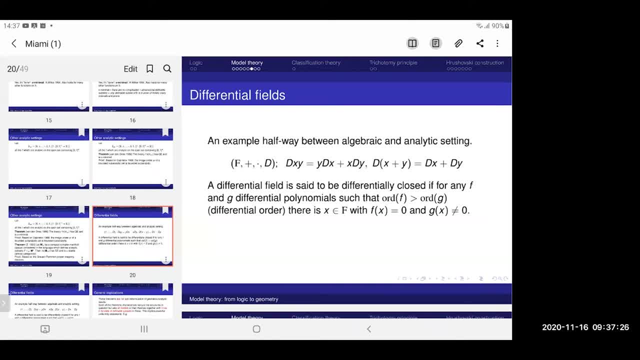 it is just one differential operator, but it is equally well works with several differential operators, but you have to assume that they are commuting, They commute. And so here you see the definition of differentially closed field. Well, and under this definition, 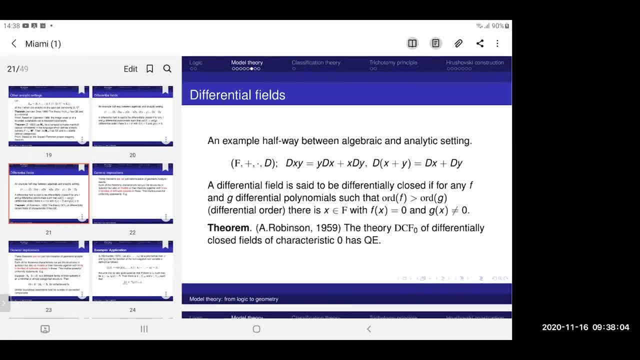 it is. Abraham Robinson, long time ago in 59, proved that the theory of differential closed fields of character, characteristic zero, has a quantified elimination. So you can say that it is state. It's interesting that at that time so the whole idea of tameness was this: completeness. 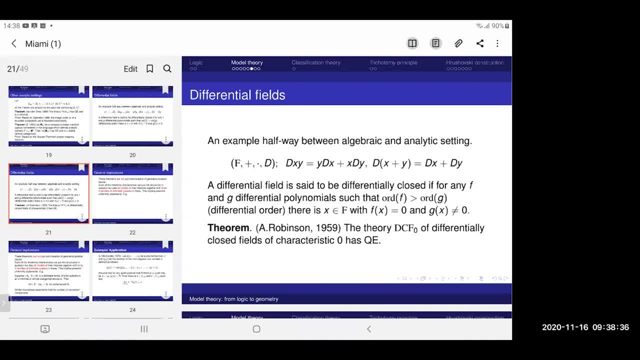 and quantified elimination. But it turns out later that people continue to to prove some nice tameness property of the same structure. So it was later proved by Lenore Bloom that actually this object is also stable And so it has a stable theory. 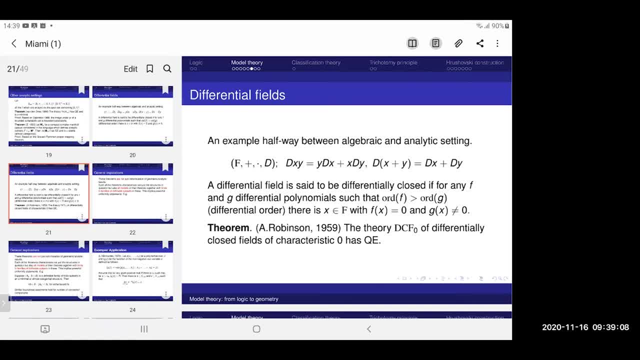 So it means that, well, generally. yeah, I'm not going to give this precise definition of stability, but the idea here is that it is a kind of tameness that you see in absolute algebraic geometry, So algebraic geometry over algebraically closed field. 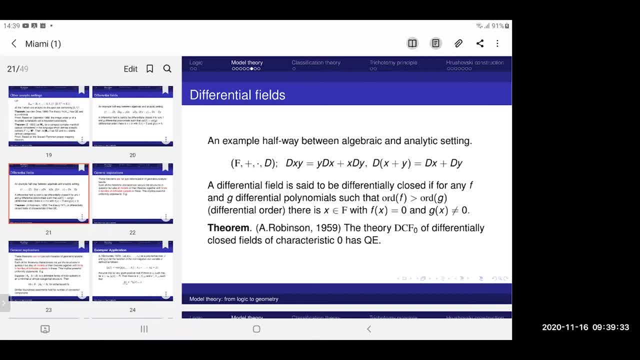 like complex algebraic geometry, Unlike the case real algebraic geometry. So the difference is that in complex algebraic geometry the properties are global And in real algebraic geometry it is. it can be different, So definable set can be different or set. 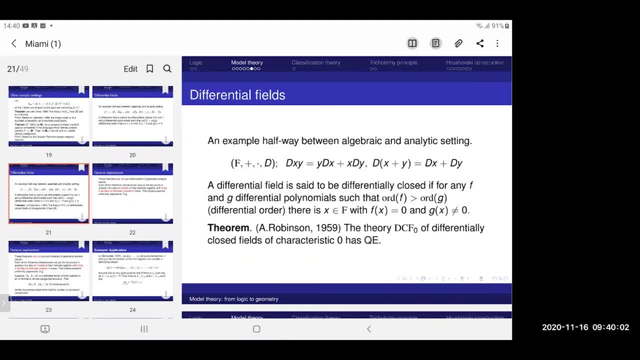 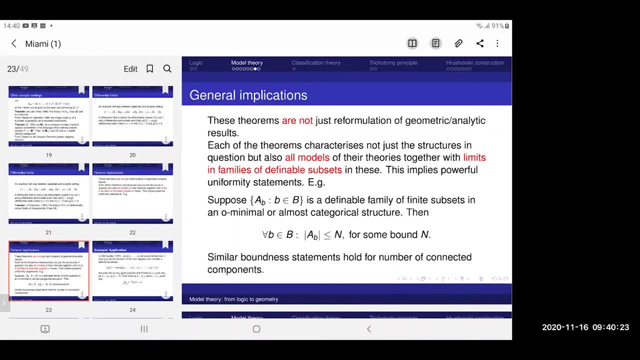 which is defined by equation- Well, especially the equation that involved this, analytic functions can look drastically different in different ways. So that's one of the implications, Okay, And so now I have come to formulating some generally implications of this, this, this list of results. 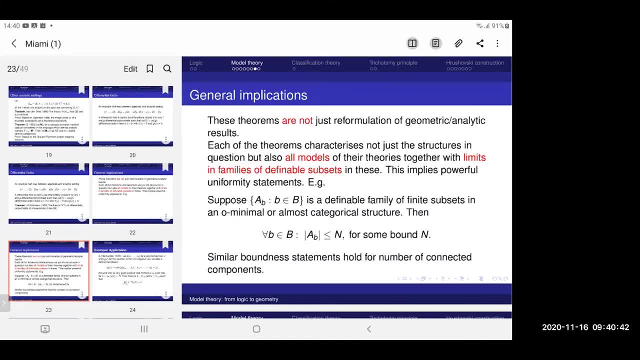 So most of them in the 1960s, 1970s. So, so, so this, this the the, the proofs you you might you might get an impression that it is just a reformulation of theorems. 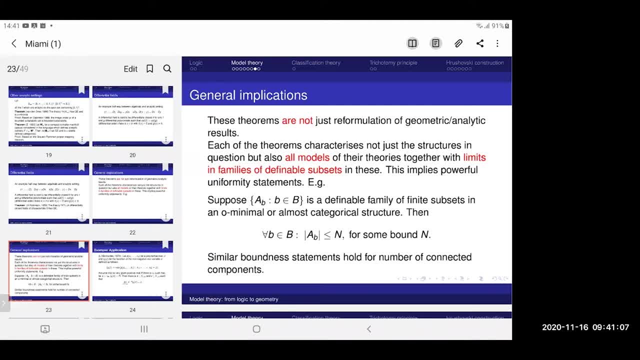 like Grauth-Kramer theorem or Chevalier theorem, just this, But it is not. It is when, when you prove this theorem, you you also systematically characterize all models, including what what we call non-standard models of of the same theory. 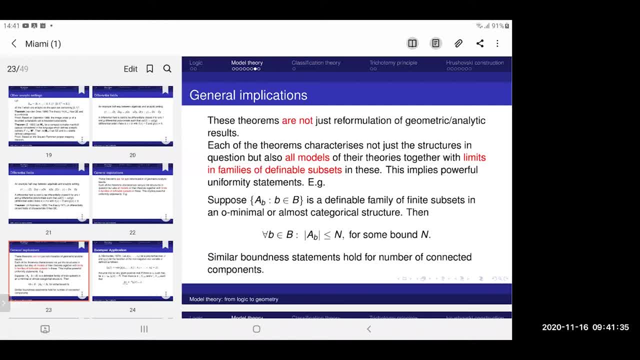 So, for example, when you work with the reals or complex numbers, non-standard models, they they can contain the, the infinitesimals. So you you do understand a lot of things about what happens in this extended world with infinitesimals. 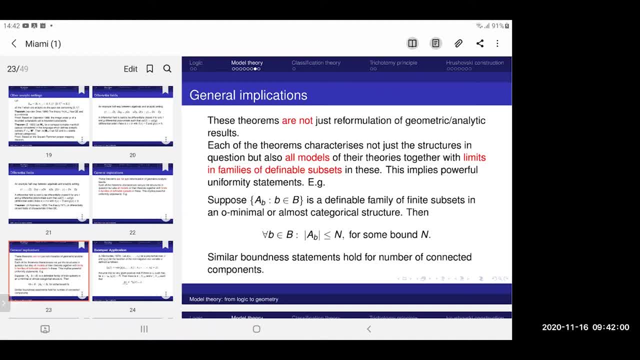 And so so this non-standard models you actually do construct through some kind of limit, limit processes, a limit process which, which, which, which, which technically is is, is consider considering ultra-product of of existing models. 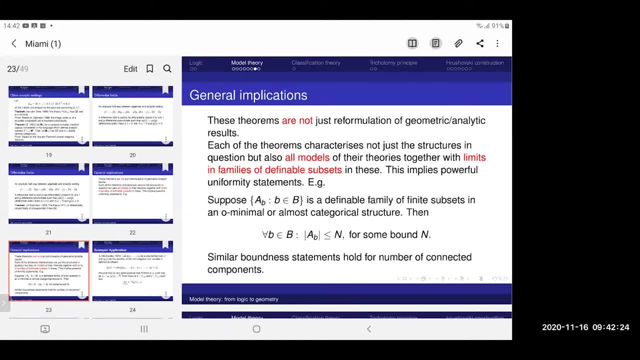 You can start with one model and then consider ultra-product of copies of this model, And, and so you have to deal when characterizing those models, you have to deal with limits And- and you do understand, by proving, when proving this theorem: without this you cannot. 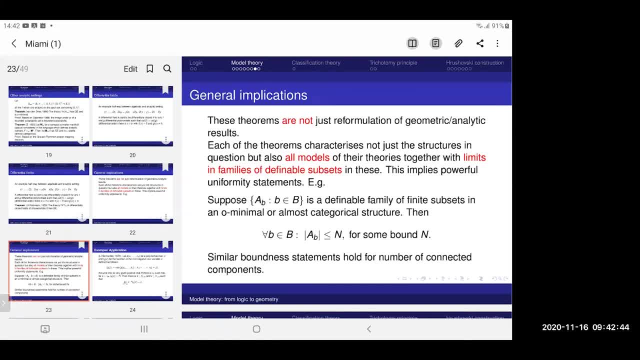 prove the theorem that you do understand limits in families of definable subsets And- and this implies uniformity statements, And here you see one of those uniformity statement: that if you have a family of, if you have a definable family of finite subsets, 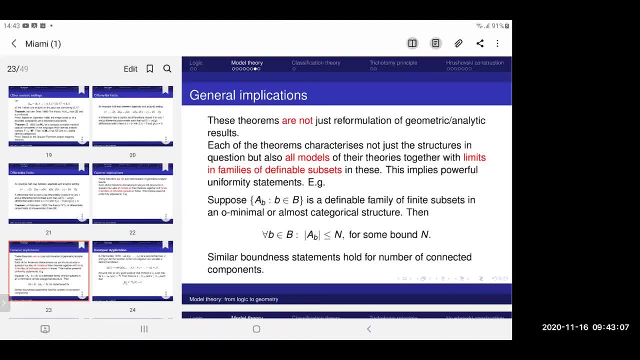 then necessarily there is an upper bound for the size of this subset. Now, if you work in a structure which has a well-defined notion of connected component, then similar is true also for the number of connected components. This is, for example, 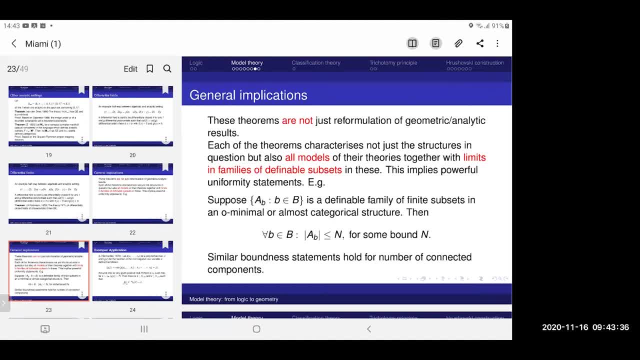 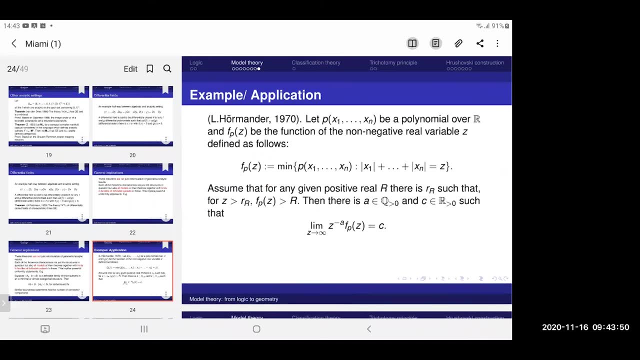 Havansky theorem for exponentiation, And so so these are the useful implications, but now I want to present here one of the earliest examples of applications, And this is application of Tarski-Zeitenberg theorem about reals. just just, you know reals. 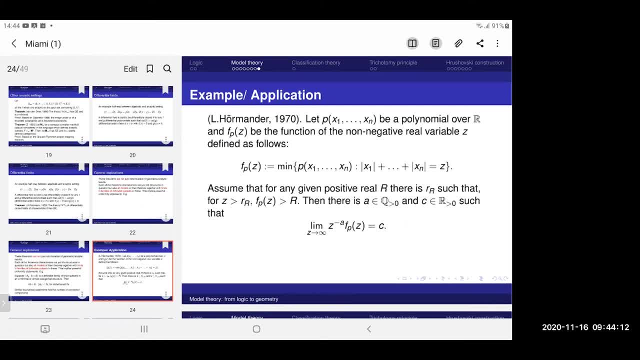 The field of reals. So it is Lars Kjormander. So you see the formulation. We look at the polynomial in n variables of the reals And and we look at at the function that returns the minimum of of the value of polynomial when we fix the modulus. 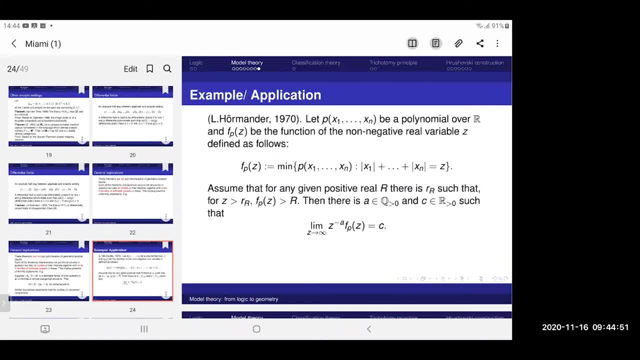 of the. the argument, Yeah so, and also assumption, is that our polynomial is such that it it doesn't take negative values And- and that is for the polynomial in n numbers, Exactly right, The F dates. So I'm speaking about the polynomial system. 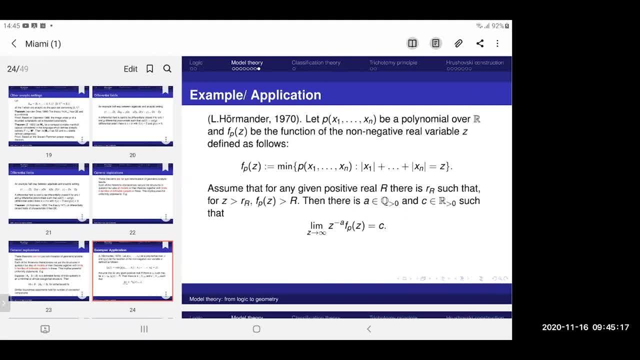 for the polynomial system and it contains, you know, a greater number of reals and a greater number of Harder levels. And so, if we assume that, if we make this assumption, that for any given positive real there is a, a bound such that over this bound, 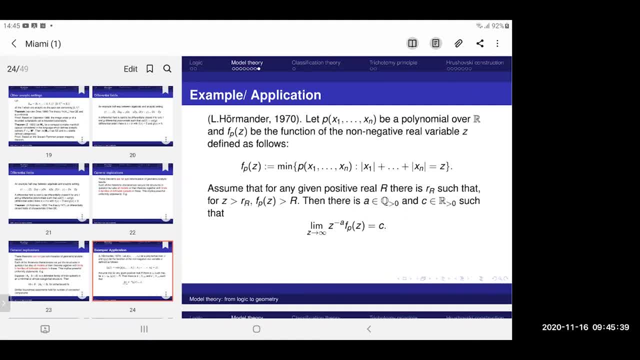 this initial real, then then actually we can, we can determine very nice the, the, the, the limit form of, of, of this function And- and this is this is this is quite important in, in the theory, 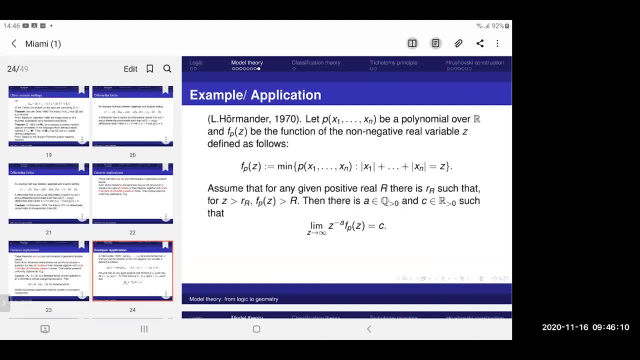 Actually, I learned about this, this, this theorem, when one of my colleagues, a professor in stochastic analysis at Oxford, approached me and asked to to clarify this, this theorem. And so I went away, thought a little bit and then returned. 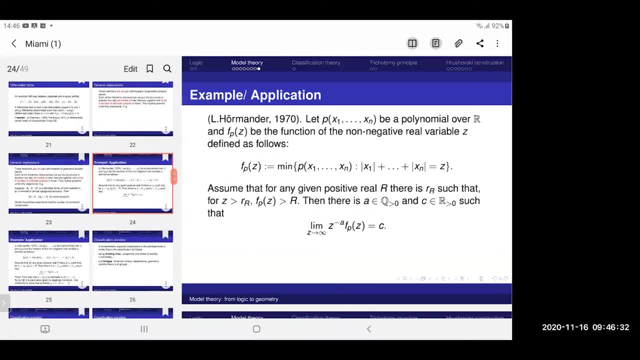 And I realized what, how to prove it. And it is very direct consequence of Tarski-Seidenberg. So the the crucial point in all this is that this function, this, that fb of z, the, the function that is given to us in this, in these terms which do not that doesn't look very algebraic, these terms because 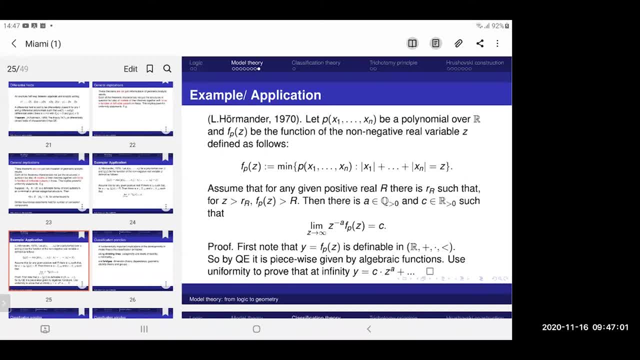 well, in fact it is, it is definable. See well, we do define it in, in, in, in, in some informal way. Well, we, we, we have to use these words which is not in our language. 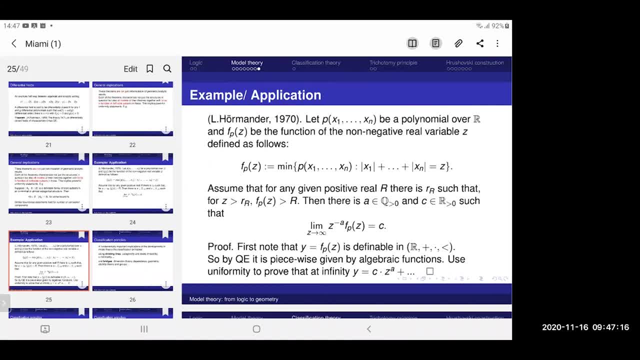 We- I mean not in our formal language- we- we need to say: it is minimum between this, that such and that have this property, and so on, satisfy this equation modulus, and so on and so forth. So if you, if you look at this, this is a very good exercise for beginners. 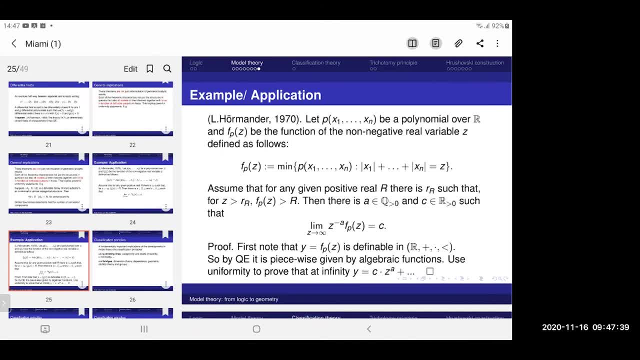 students. we often give them this exercise, this sort of exercise. Well, but you it? it would require to use quantifiers. You will. you would have to say: there is a value such that every other value is over this, and so on and so forth. 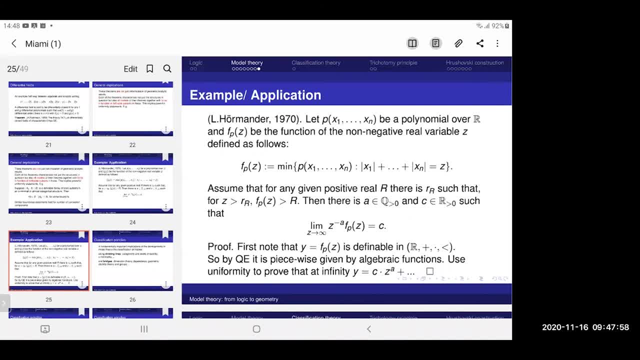 So it is. it is really an expression that is is quite long and heavy with, with quantifiers in it, But it is definable. This is the the main thing, And then the Tarski theorem. 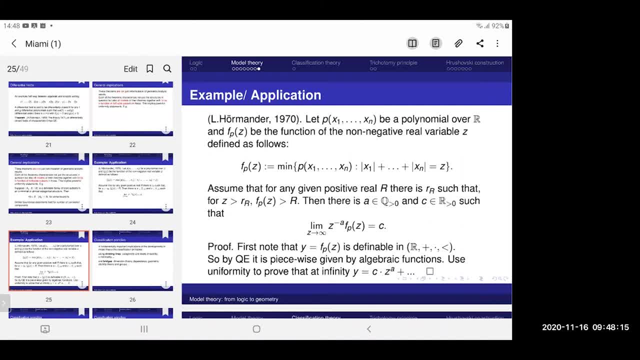 Tarski-Zeigberg says that it is equivalent to very simple expression And so this function is piecewise, is given by algebraic functions, But more exactly it is. it is not just a piecewise seal. You can use this uniformity that I 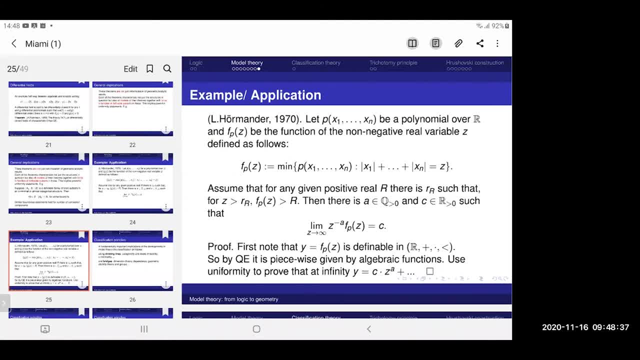 I mentioned, to see that it has this form: y is equal to a coefficients time, z to power, a, where a is some rational number plus lower terms, And and that's it. So so this is a beautiful 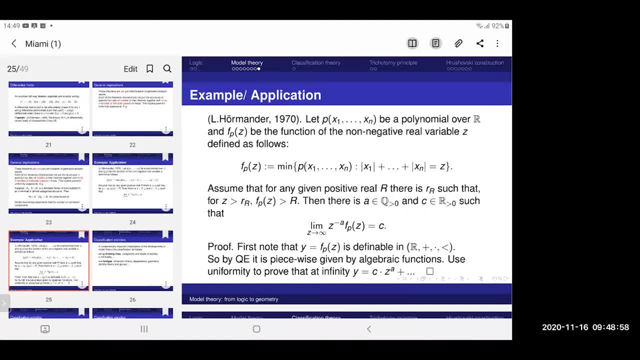 application: And, and, and. so this is a beautiful application of one of the basic theorems, of very simple things. So we shouldn't be surprised very much that you know when you, when you prove, prove similar theorems for: 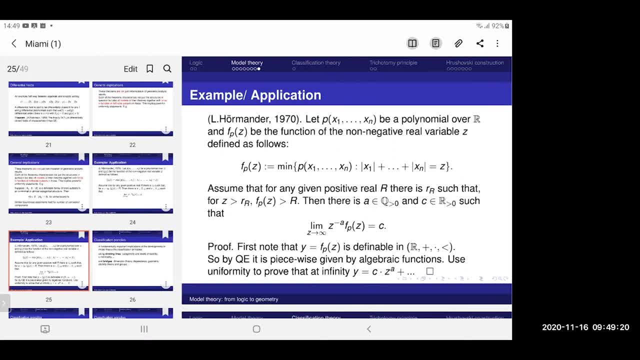 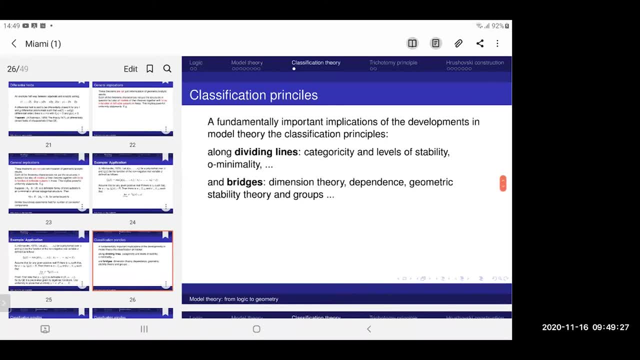 things that involve exponentiation, then that's that's much more powerful, has, has a potential much, much bigger. Okay, So, from from all this experience we do, we come to, we arrive at following classification principles: 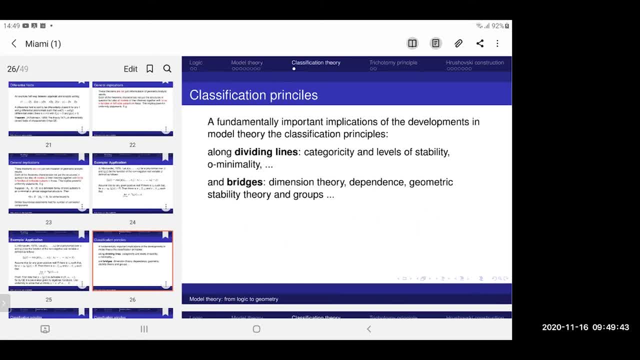 So so we we can classify, in fact, the, the structures, we we now look at structures as being part of some classification matrix where we have dividing lines like categoricity and these levels of stability. 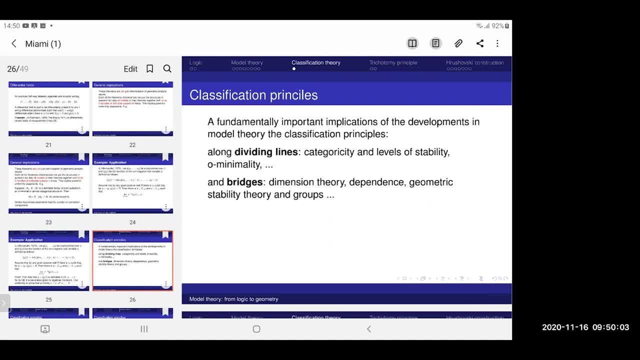 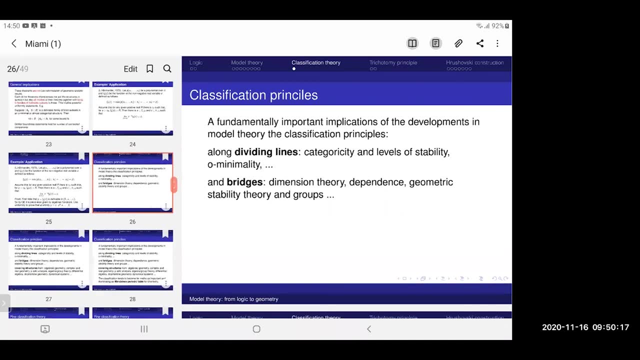 or minimality. there are other forms of this. And then the bridges between these different levels are this: dimension theory, dependence, geometric stability theory, the theory of groups in these structures, and and so on, And and. 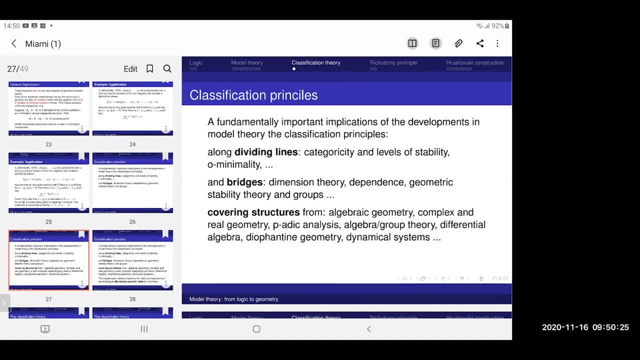 for example, there are there are literally dozens and hundreds of examples from algebraic geometry: complex and real geometry, biaeric analysis, algebra, differential algebra, diction, geometry, dynamical systems And yeah. 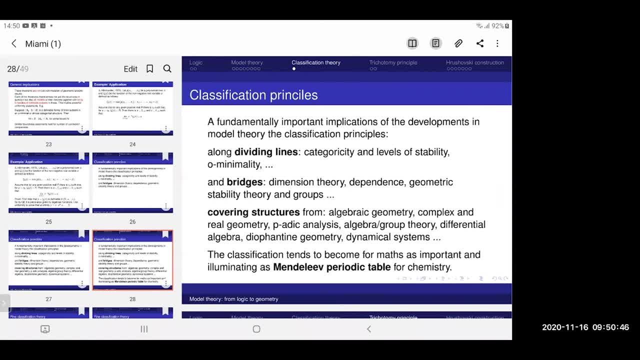 I, I, I like, I like this thought that, in fact, the way that we now think about this classification theory- It is, it is like for mathematics is- is as illuminating, it has a potential to be as illuminating as Mendeleev periodic table. 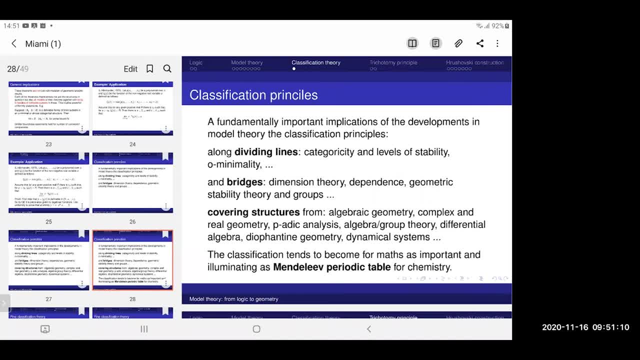 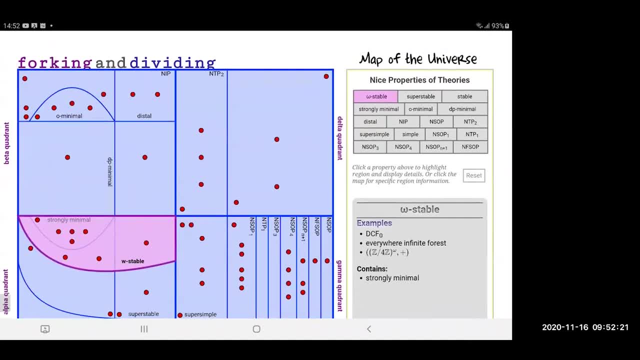 for chemistry. And let me show you. on the internet there is a site. this is a site where I'm learning by some of my colleagues. So you have this map of the universe of. so you have. you know that. that's the way we are thinking about. the universe is populated by. 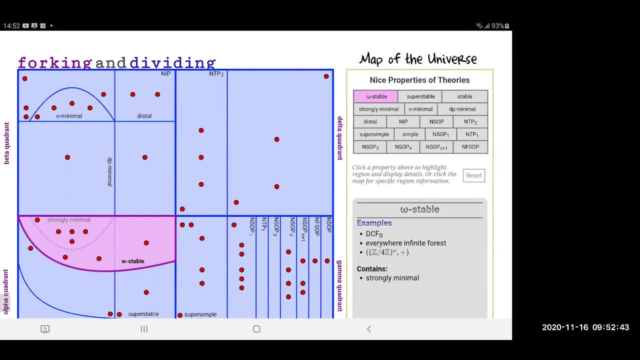 various mathematical structures, And, and you you see here. so so, so. so here we come into the world of minimal structures. If we pressed this one, oh sorry, yeah, I pressed the wrong one. So so here you see. 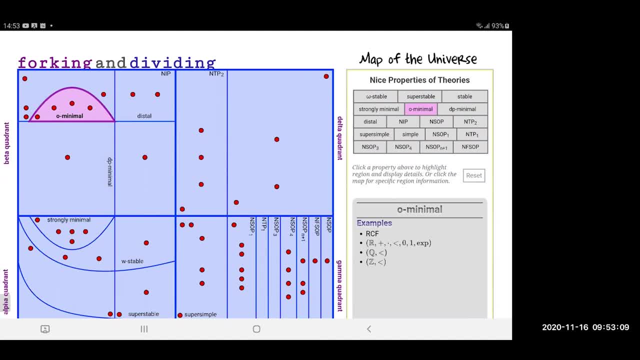 on the right, right low corner. you see that we have this real closed field that we just talked about as one example. then we also have the field with exponentiation, and then there are some, some other examples. Now if we have, if we go into this corner, that 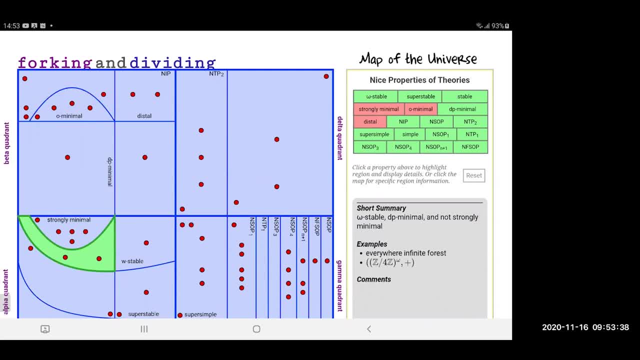 we see some, some, a lot of other structures with other examples. So here are what we call strong, minimal structures, So algebraically closed fields and vector spaces and so on, And and then then in the then. So we have, as you see, on the left, we have all minimal. 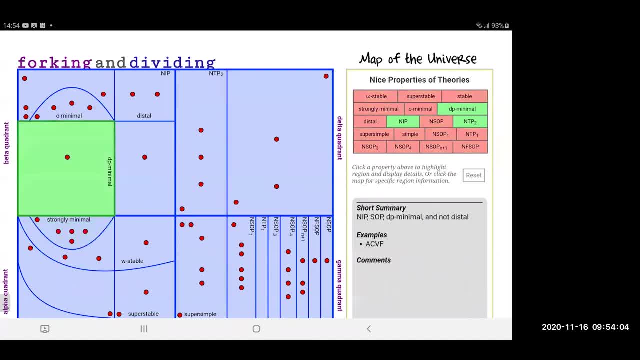 we have strongly minimal. So here we have so-called DP minimal and various kinds of this, And then we have various kinds of stable structures and super stable structures, And so, again, if you look at this DP minimal, DP minimal, what you see in the right lower corner, 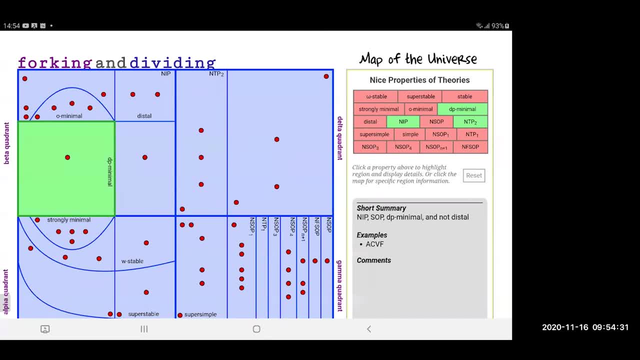 so there is this very important example. So the abbreviation for it is ACVF- it is Algebraically Closed Valued Fields, And Khrushchev used it in very, very effective way in improving so it's. it's a lot of work around it. 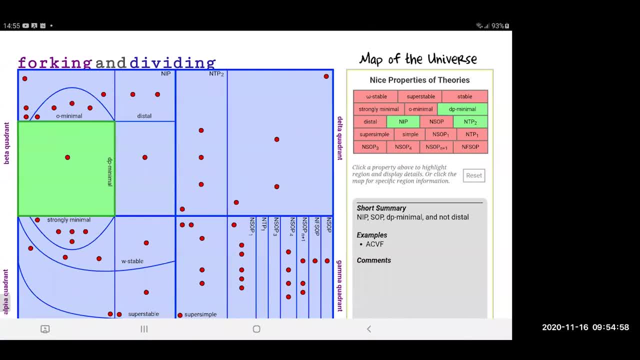 And Khrushchev and Lazare proved some, some great results in in non-Archimedean analysis, Berkovich spaces and answering some open questions. So it is so a lot of applications sit here on this picture And so that's unfortunately it is not. it is not complete. 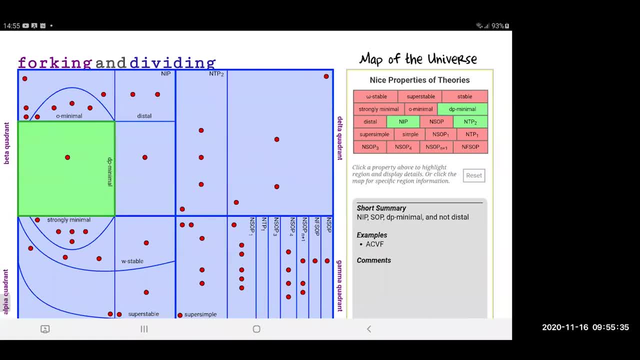 So in fact there must be hundreds of of such such objects that marked by by points here. And so it is. it is of good use to, to specialists in this, but to to make use of it for broader monomeric community, of course. 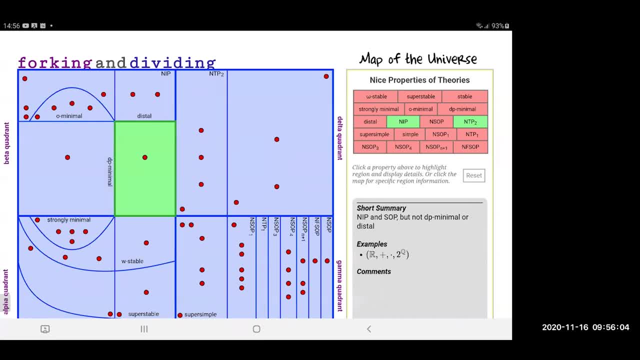 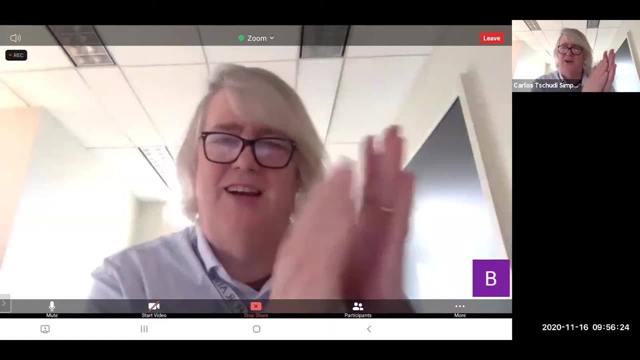 it. we should put in much more of known examples, known and useful examples. Okay, that's it. That's what I plan to present for today. Thank you very much, So I think everybody should feel free to unmute yourself. Thank you very much, So I think everybody should feel free to unmute yourself. 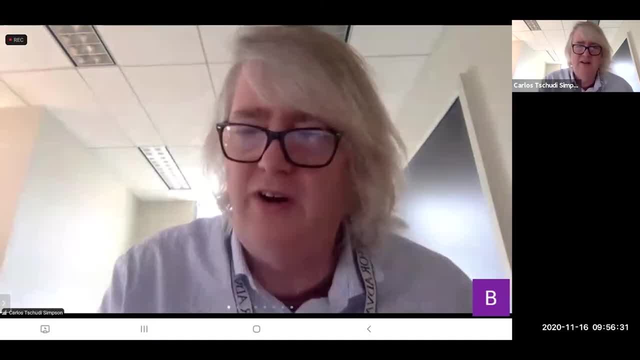 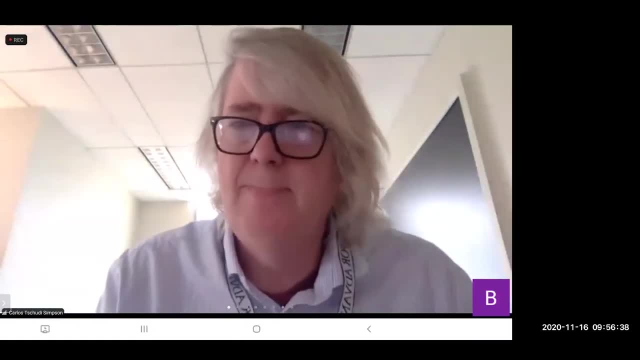 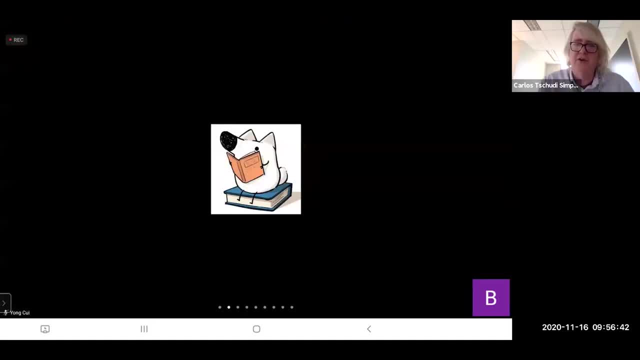 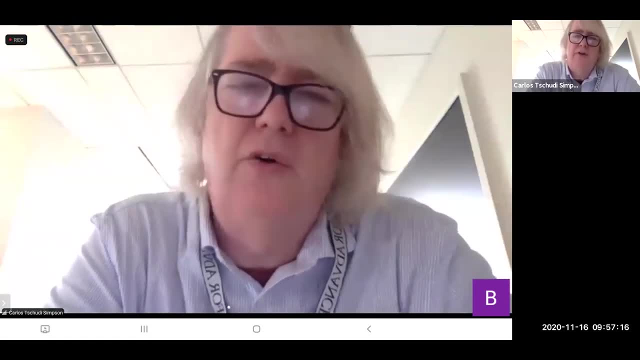 Thank you, So now? so I think we have plenty of time for some questions. So does anybody have any questions? Maybe, so maybe let me ask a question: What about other types of structures that are like, maybe less related to complex geometry? 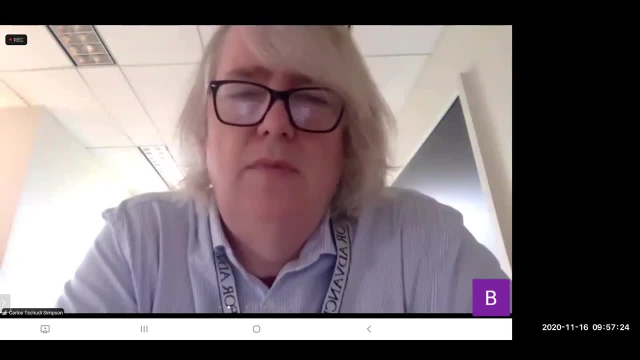 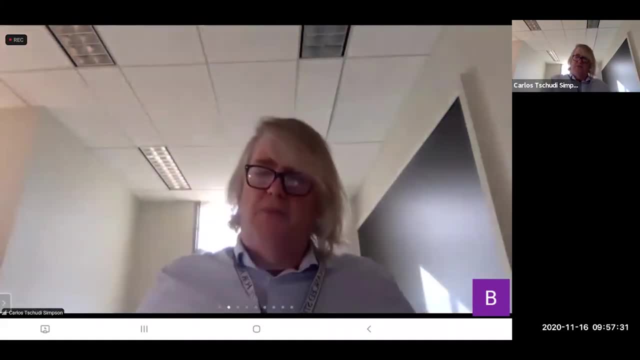 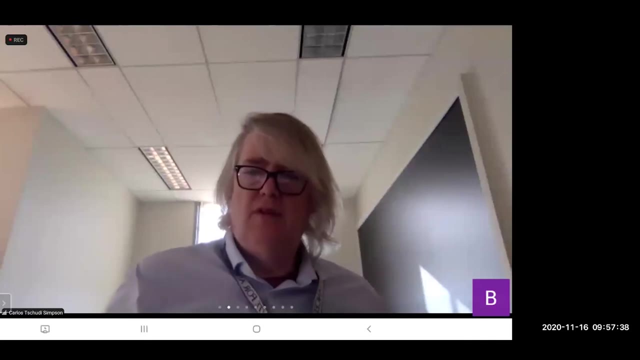 What do you mean? other other, what? Well, maybe are there similar types of things that are happening, but without the real numbers, for example. Yeah, well, it is as I said, you see, it's. so you have this. 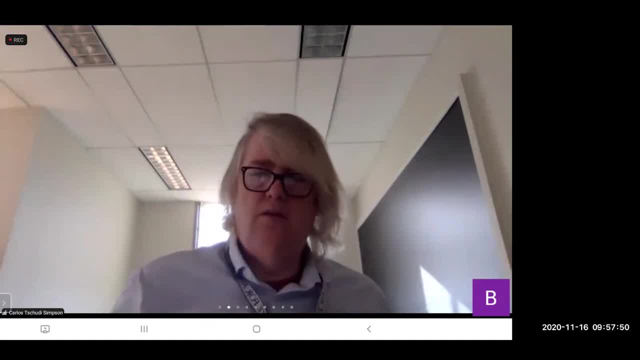 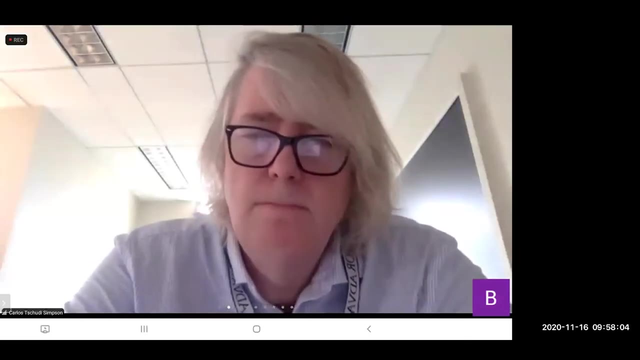 these different boxes in this classification theory, And so it is different degrees of tameness in this box boxes. So, depending of course on so, for example, in non-Archimedean analysis, you would, you would, you would have the P-addicts.